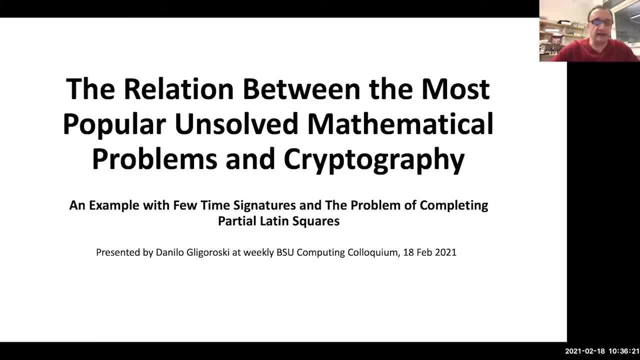 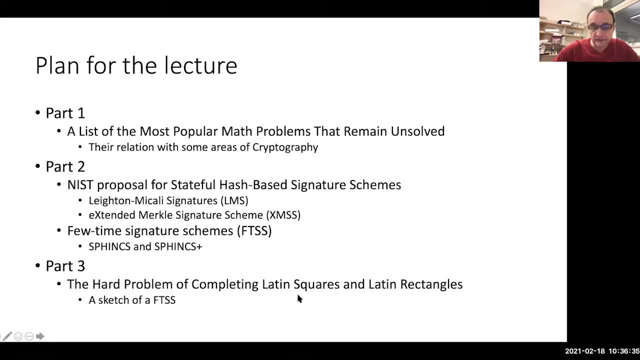 are the possible pathways to apply whatever I'm doing in a nice and interesting field of my area of mathematics. So several years. this is the plan of the lecture. The first part actually will be related with one article that I read one and a half years ago in Popular. 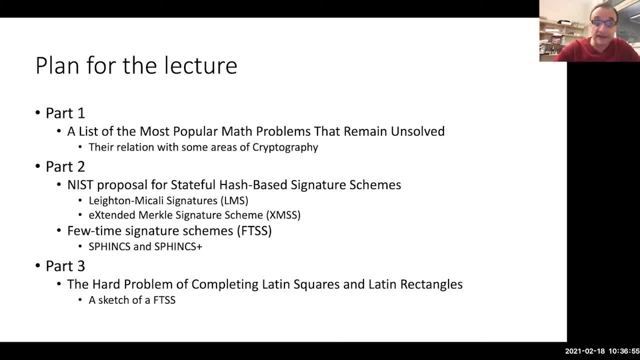 Mechanics, but it was about the list of 10 most popular mathematical problems that remain unsolved, And since when I was reading that, I actually work in cryptography and I wanted to talk about that, So I noticed that actually the first seven topics are somehow related. 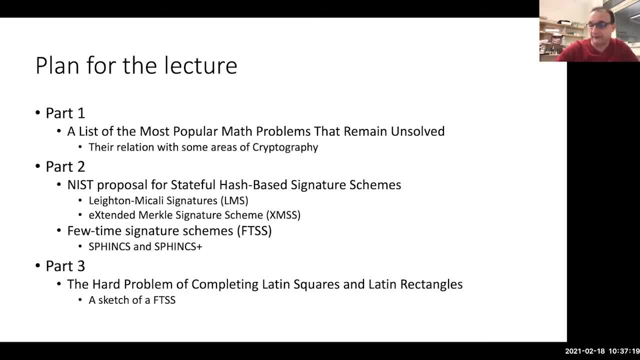 with one very applied mathematical field, which is the cryptography, And the second part will then mention one thing that maybe it will be for the audience, maybe a little bit far away, I don't know- but it is about one ongoing standardization process of the 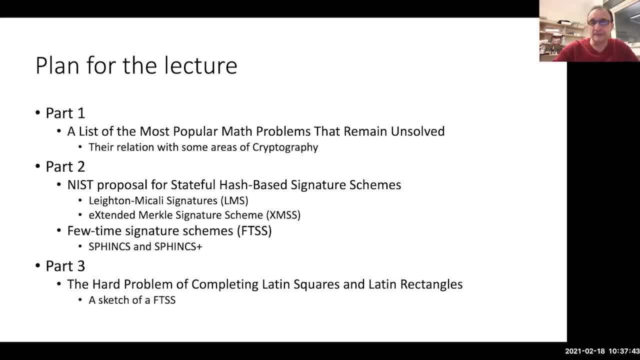 National Institute of Standard Technology from the United States about one specific so-called stateful hash-based signature schemes, And then to connect the part one and part two, I will again mention one hard problem which is completing the problem of completing partial Latin squares or partial Latin rectangles, and how it can be actually connected with. 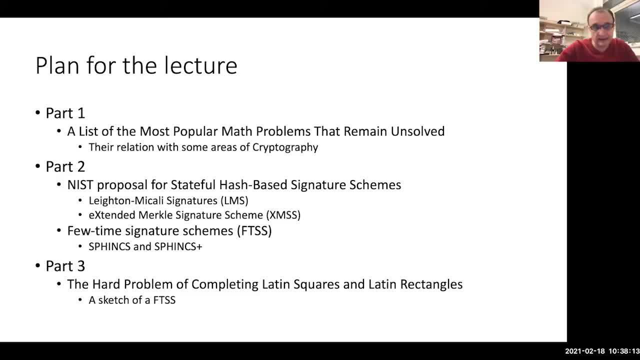 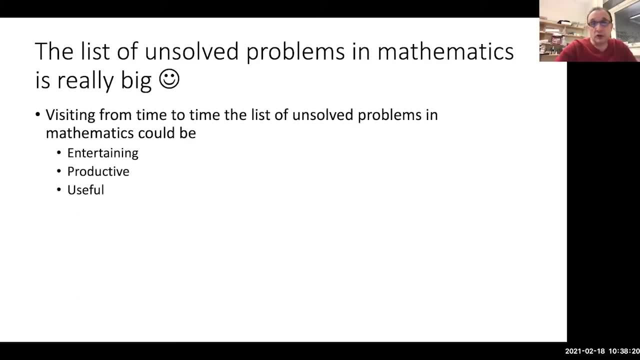 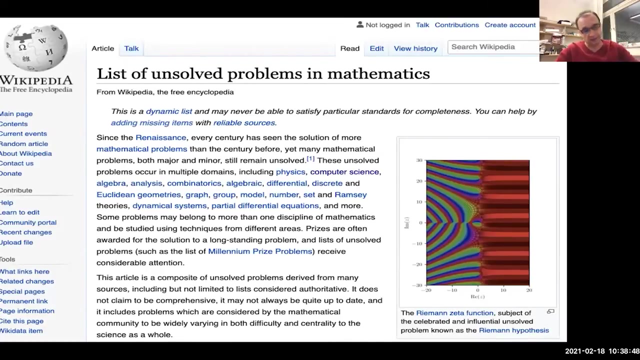 some of the first and second part of the talk and that's the plan for the lecture. So the list of unsolved mathematical problems is really big And today I will mention just 10 of them. But actually, if you happen to visit Wikipedia, You will find maybe lists of hundreds of unsolved interesting problems. 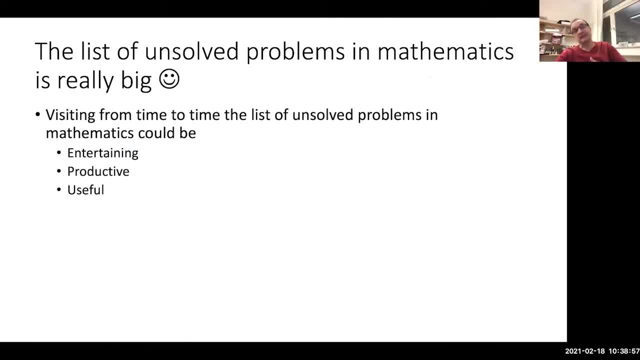 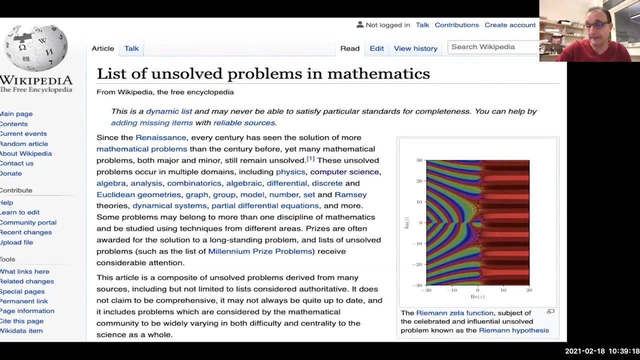 and well visiting. from time to time this list can be personally entertaining, but also it can happen that you pick up some idea or even interest And at the end it can turn out to be useful, And these problems varies from different areas of mathematics. 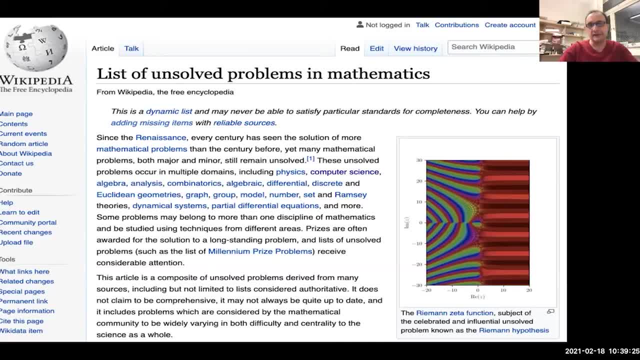 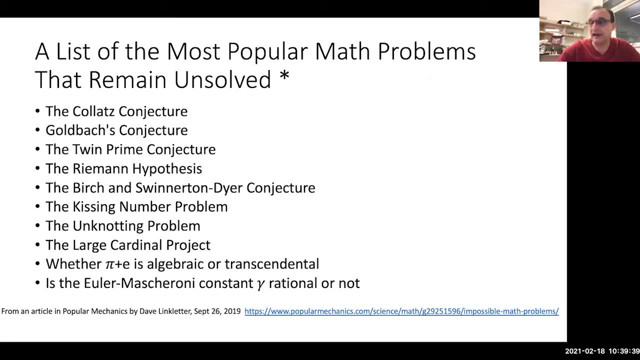 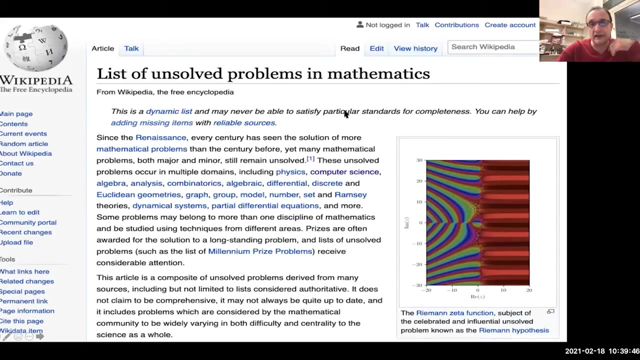 algebra, combinatorics and many, many other sub areas and disciplines of mathematics. So, as I mentioned, this list is arbitrary or you can compose probably your own list And, as this actually in the beginning, if you visit Wikipedia and this list of unsolved problems, 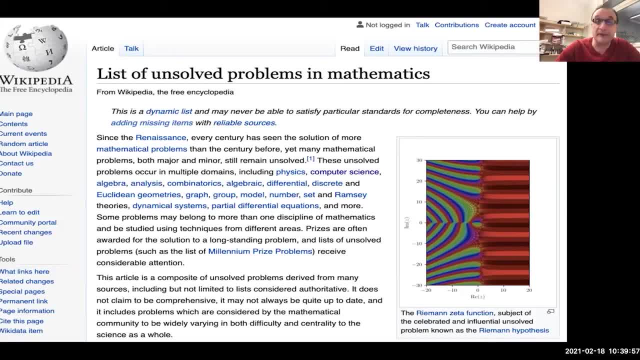 actually it says right from the beginning: this is a dynamic list and may never be able to satisfy particular standards for completeness. but maybe you can even add some of your unsolved, some other problems that is not mentioned on this list. So again, this list from this article. 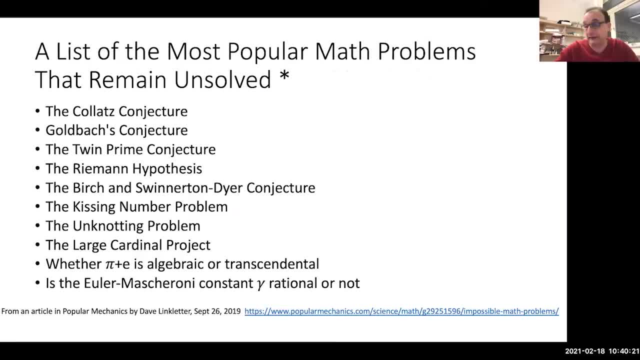 from Popular Mechanics. actually, of course, that might not be according to your specific mathematical discipline that you are working on, maybe according to your taste, but still it was provocative for me, but still it was provocative for me, but still it was provocative for me. 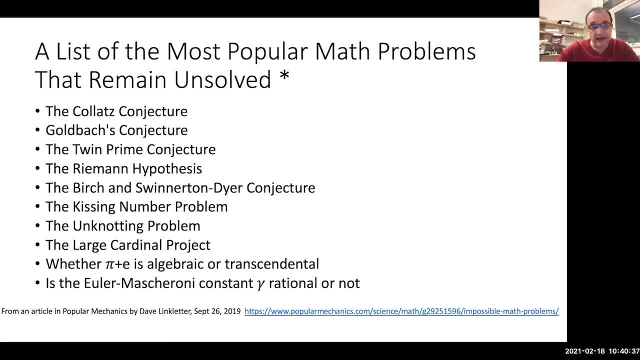 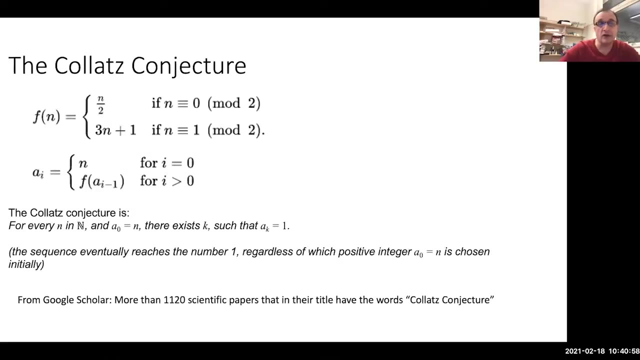 when I read this article And as I mentioned at least the first seven problems, there is a connection with cryptography and, as I will briefly mention that connection, For example the first one, the Collatz conjecture. well, maybe you played a little bit, even in high school. 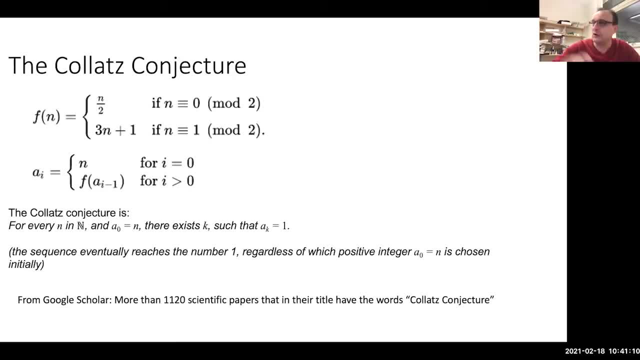 I remember when I was in high school, on the whiteboard or blackboard we would discuss, and some of the classmates brought up this one. So imagine that you start with whatever number and then, if the number is even, you divide it by two. 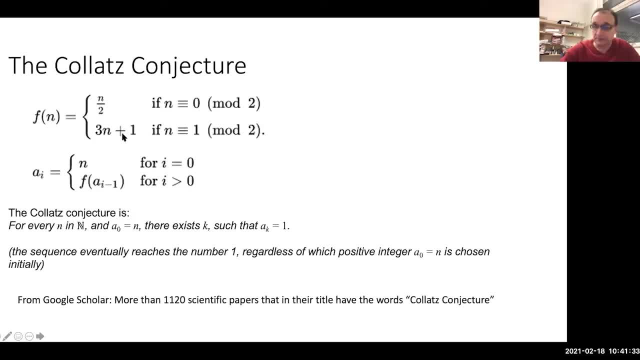 but if the result is or you multiply the result by three, add one and continue that process And eventually every sequence will end up with the number one. So it kind of captures the. is it? wow? is it unexpected? Look, I'm dividing by two but I am multiplying by three. 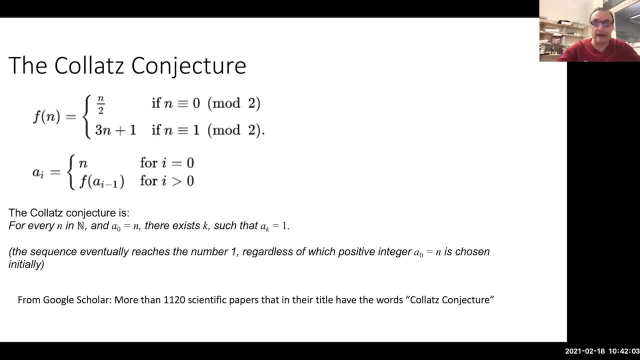 I am increasing even faster than I'm decreasing, but eventually you end up with number one. So, and there is a long list of nice work that actually are advancing the discipline and the knowledge about this problem. But how can we, since I'm working for a long time in 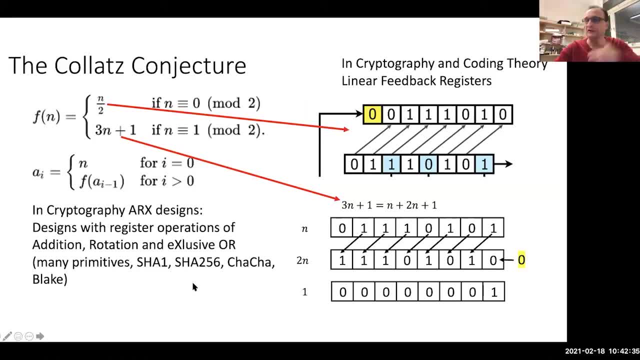 a cryptography designing hash functions or stream ciphers or something. in cryptography and encoding theory we have so-called feedback or linear feedback shift registers. So if you have a number N, you can represent it binary with zeros and ones, But then when you do this operation, dividing by two, 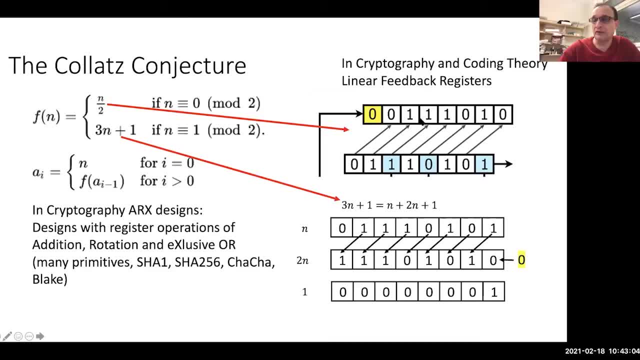 actually you are just shifting it And since it was even number, it ends with zero at the least significant bit. So you just shifted to the right for one position, add or inject one zero from the left, And that's the result. So that's the result of this operation. 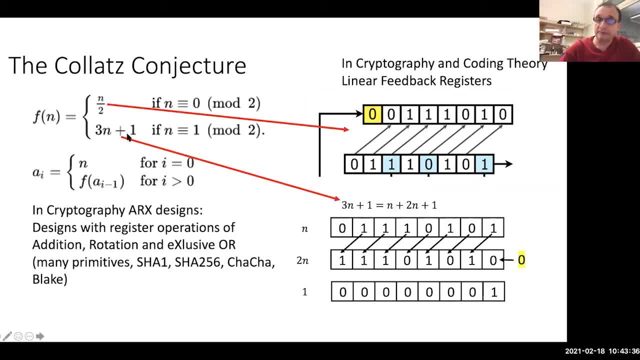 Well, what about the other operation, Multiplying three plus one? Again, you can. if you represented your number N as a binary register, well, first you just look that yeah, actually this three N plus one, you can represent it as N plus two, N plus one. 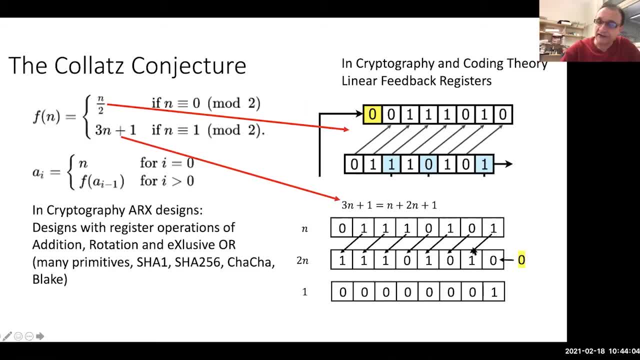 So N is zero. This is your original register. Then you shift it, But actually now you're shifting and moving it from the opposite direction than this division by two. Now multiplying by two is just shifting everything to the left and injecting zero. 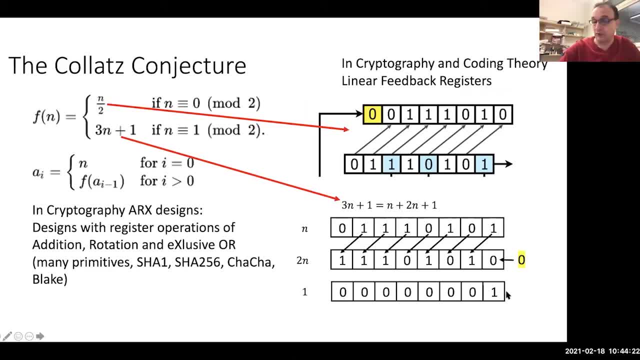 And then one is just a register with all zeros except that least significant bits, And if you add, but now the adding is with this, as we know, this symbol with the carry, with the carry sign, Basically this composition and these operations. 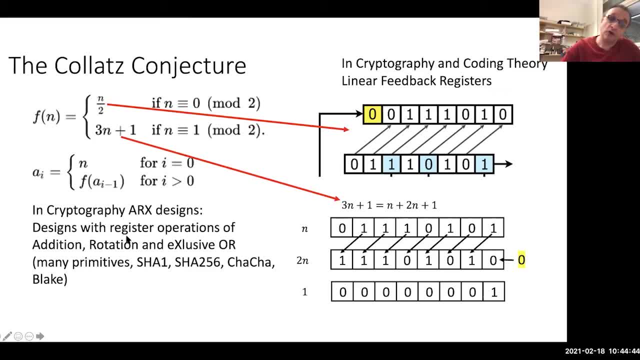 are very well also known in cryptography. Those are so-called args design. So the current hash standard used in so many operations, so many protocols and other more complex primitives, the hash function SHA-256 and the previous standard SHA-1 and many others primitives actually are using this. 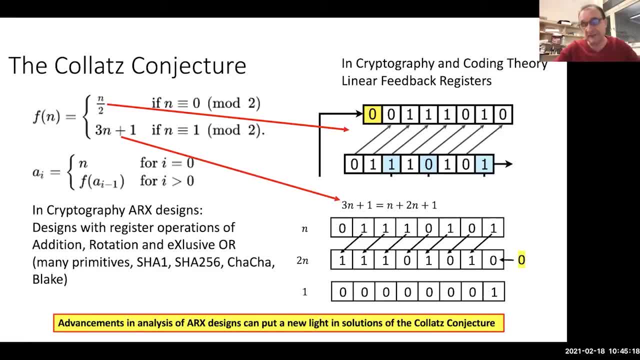 So basically, the advancement in analysis, so there is a analysis of these designs. The advancements in analysis of arg designs actually can put a light in the solution of color, call it conjecture, and vice versa, And there are some works which actually make that connection. 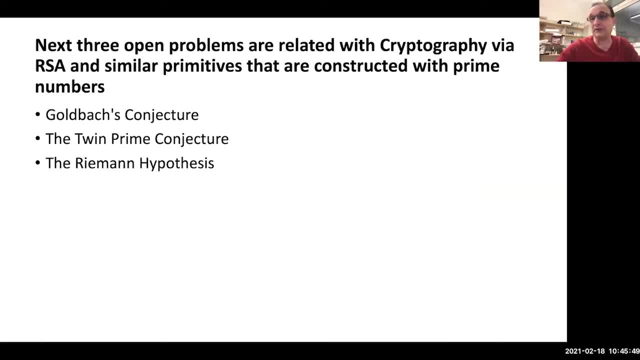 The next three open problems are related with cryptography, but from the number theory perspective- and probably you have heard about RSA, public key algorithm that is constructed with prime numbers- And the next three famous mathematical problems: the Goldbach conjecture, the twin prime conjecture. 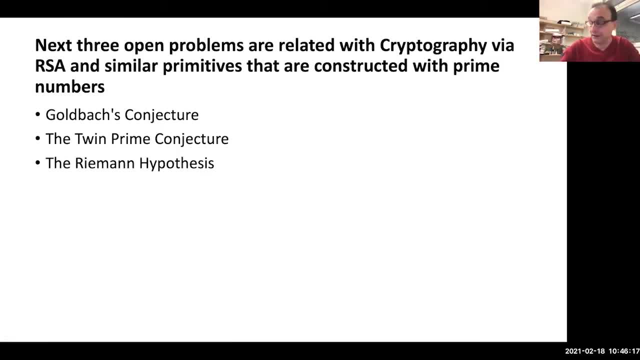 and the famous Riemann hypothesis actually are in connection with prime numbers. There are many others problems, but at least this. they were not mentioned in that popular mechanics article, but at least these three are in connection with prime numbers. So Goldbach conjecture. 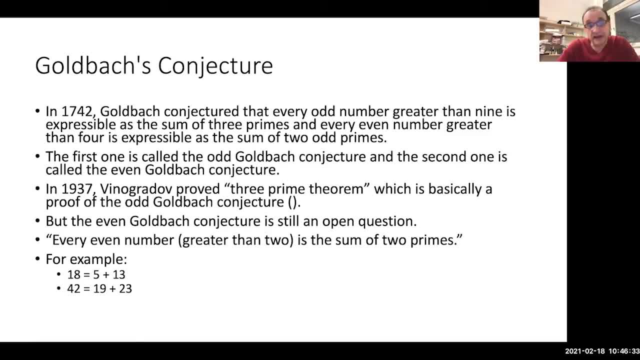 in 1742, Goldbach conjecture that every odd number greater than nine is expressible as a sum of three prime numbers And every even number greater than four is expressible as a sum of two odd primes. The first one is the odd number. 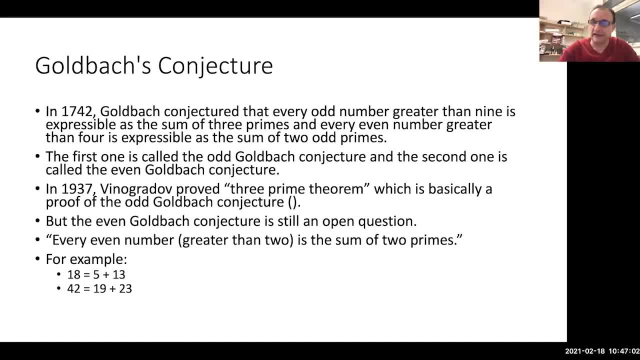 that's called the odd Goldbach conjecture, and the second, the even Goldbach conjecture. Vinogradov, a long time ago, in 1937, proved three prime theorem which basically is the proof of the odd Goldbach conjecture with some refinement. 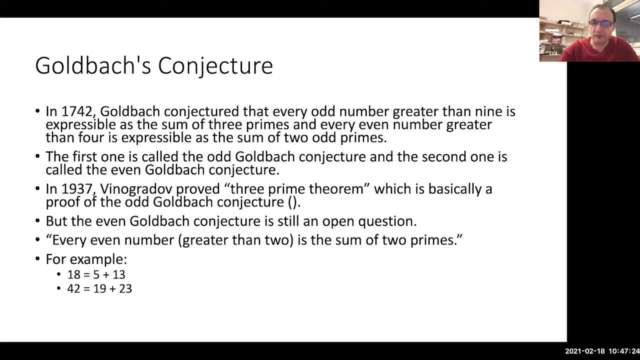 but basically it's the proof of the odd Goldbach conjecture, of the odd global conjecture. But the even global conjecture still remains an open problem. For example, 18, you can represent as five plus 13,, 42, and many, many others. 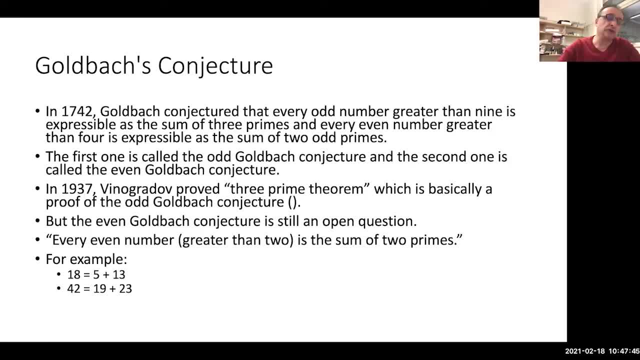 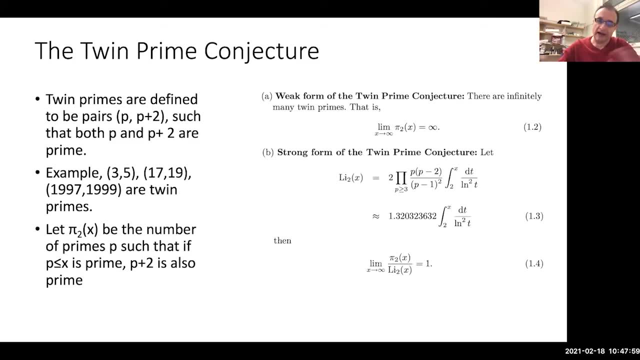 Actually up to 10, to the 15,, I think, by modern computers. it was checked and it holds. But there is advancement, And so I will speak why those are advancements at the end of this three mentioning of these three problems. 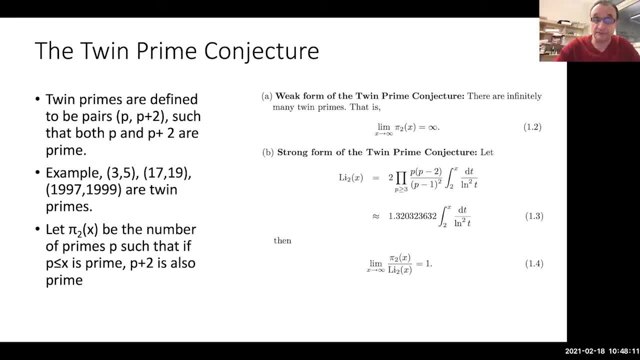 The other is the twin prime conjecture. The twin primes are defined as the primes which differ only by two p and p plus two, and both are primes. Examples three, five, six, seven, eight, nine, 10.. 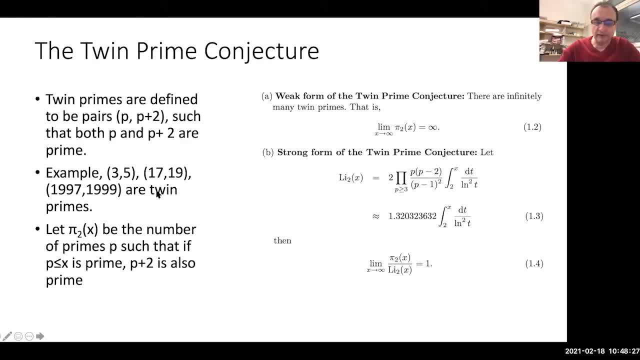 Seven, 19, and many others. So if we have this notation of pi, two of x would be the number of primes, numbers that are less than x And also for which also p plus two is the prime, Then basically this twin prime conjecture. 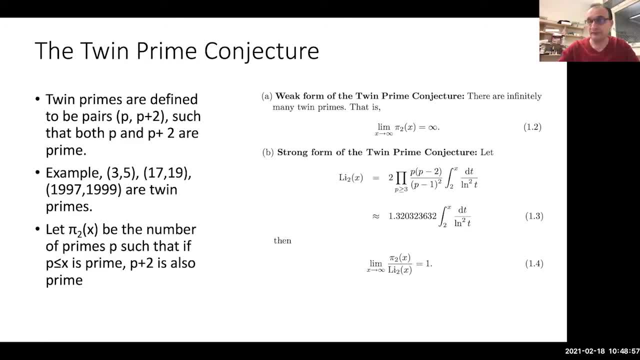 says that there are infinitely many twin primes, meaning that the limit of pi two, when x goes to infinity, is also infinity. And there is even a strong form of the twin prime conjecture that if we take the short notification of this product and the finite integral, 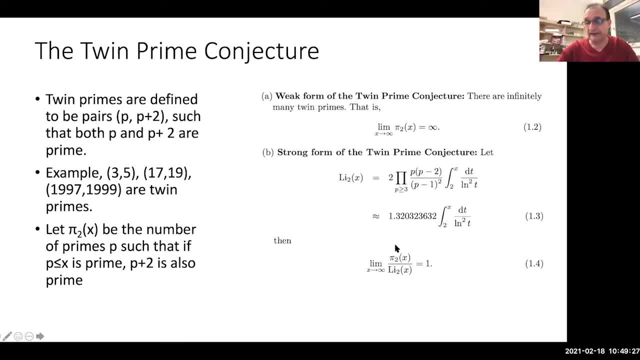 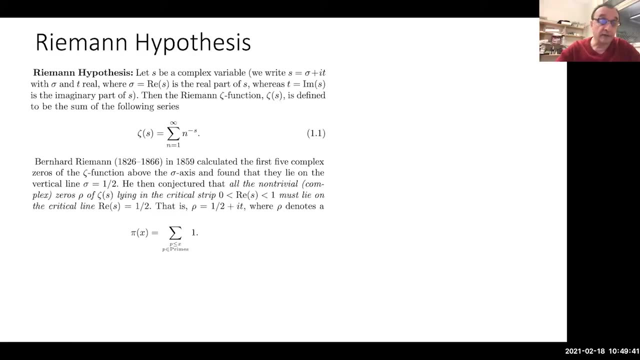 then basically it says that this approach is how this actually the number of pi two and this product actually they approach same value. And the famous Riemann hypothesis: if s is a complex variable, let's say, or if you write it as sigma, plus i t. 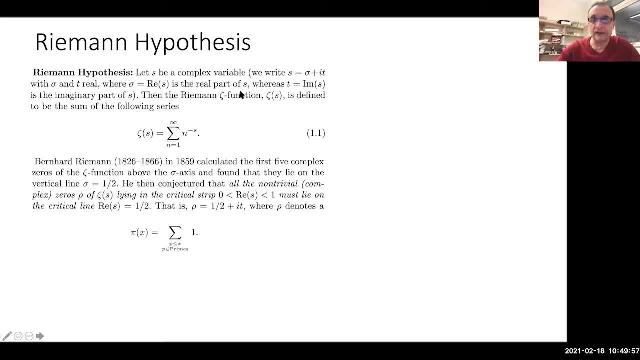 and then if we construct the Riemann zeta function that depends of s in this form, in this infinite sum, And after actually Riemann calculated the several few zeros of this zeta function, he noticed that all of them are lying into the critical line. 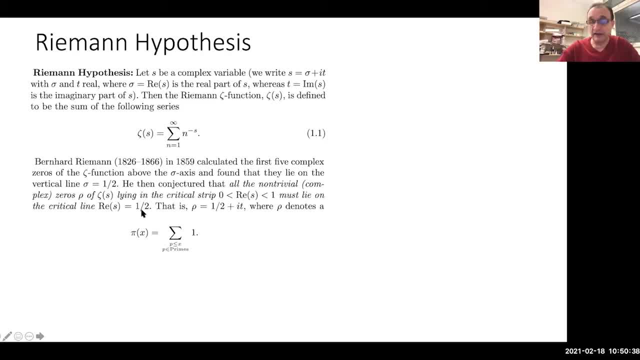 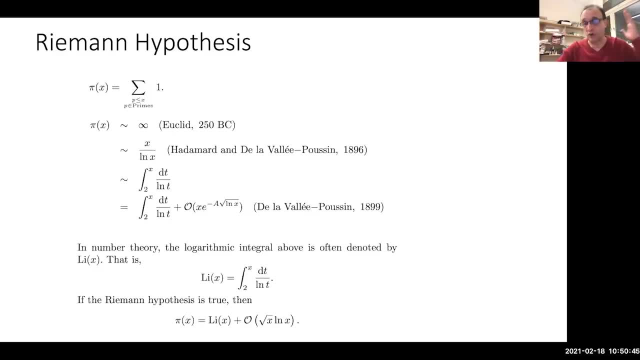 which is one half. So the conjecture is actually that all of them lie in the on that real line. with the value one half, Or with the notations that are introduced here, you can say that the Riemann hypothesis is true. 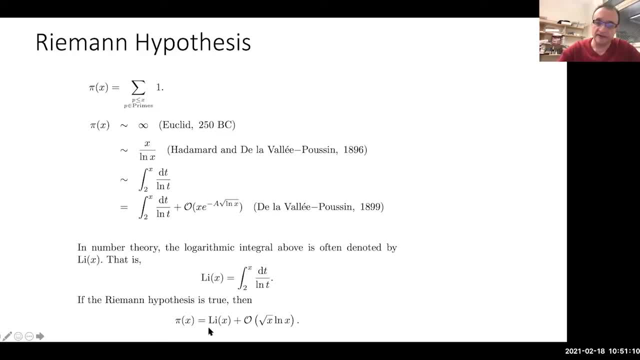 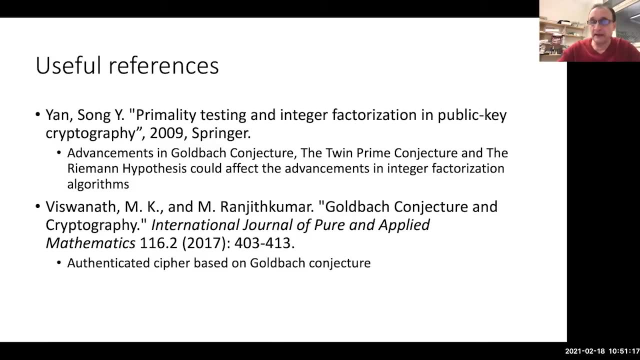 then this expression holds Now, what would be the why these three and similar open problems in mathematics would be useful in cryptography, Actually primality testing and integer factorization, if these advances actually are putting more knowledge or light into the distribution? 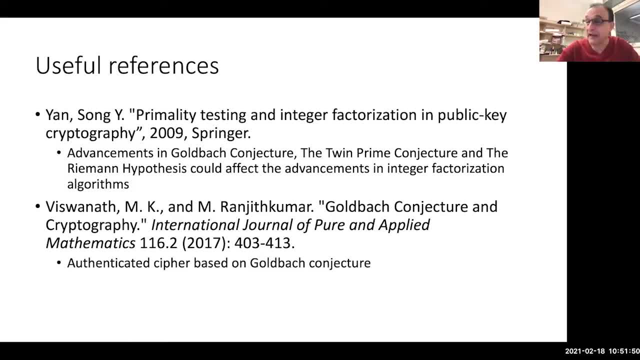 of prime numbers and the relations between prime numbers and basically those that extra knowledge can help in advancements of the algorithms that are performing integer factorization or some other type of analysis. Also there have been based on, at least for the Goldbach conjecture. 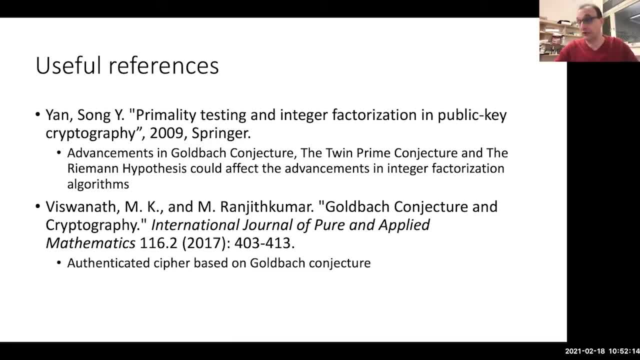 recently a proposal for a constructive, not just integer factorization in order to break some of the cryptographic schemes but to construct the cryptographic schemes based on the Goldbach conjecture. And there was this is some proposal for authenticated cipher based on the Goldbach conjecture. this reference here. 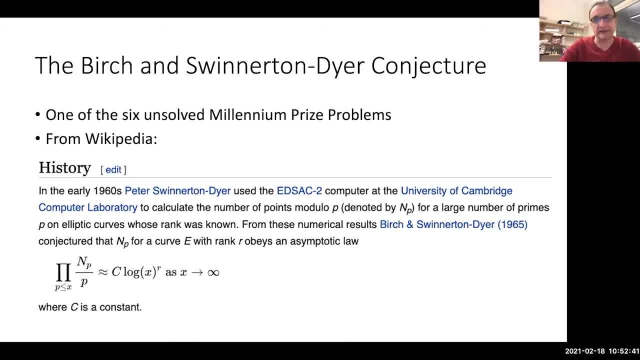 Now in connection, this Birken-Swingerton-Dyer conjecture. this is from a recent days, but this is one of the six unsolved millennium price problems and is in connection with modern or modern produce problems coming from the the. 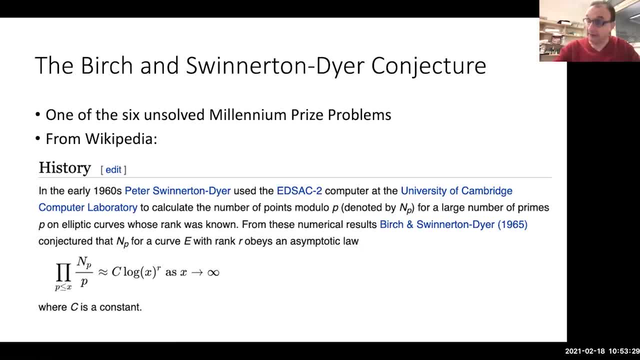 elliptical curves And basically, when the era of computers back in 1960s started to be applied more and more and mathematicians started to apply more and more, they started to count the number of certain, basically the number of points on elliptical curves. 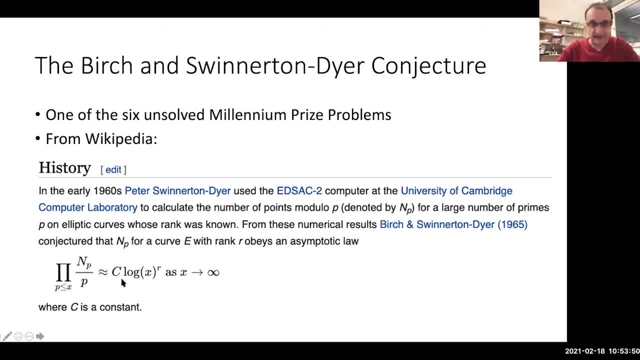 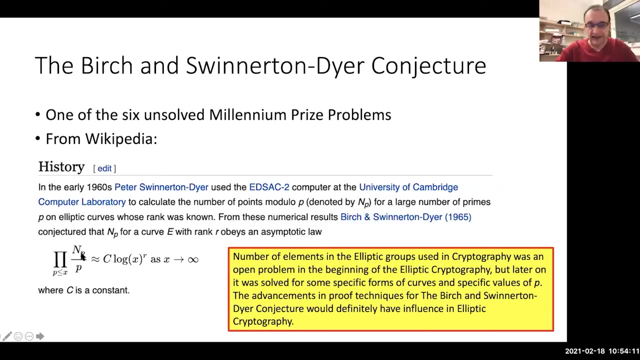 And this conjecture, basically, is that this number of points, or modulo p, modulo prime number, but on elliptical curve, if it is ampere, then this ratio or the product of this ratio converges to this expression here, And why this would be important. 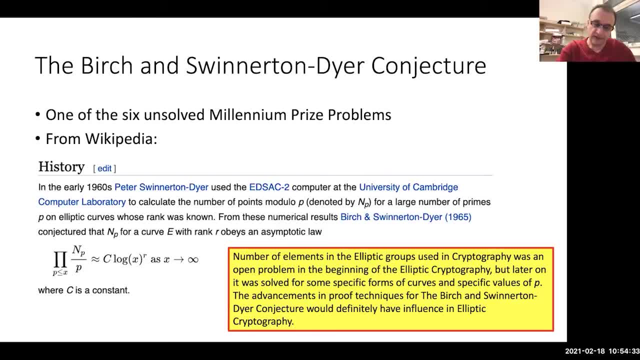 Well, in the beginning of the elliptical curve cryptography there was an open problem about how many points are on elliptical curve specifically chosen for the cryptographic purposes, how many elements the elliptic group has. Later that problem was solved, but for specific values of p. 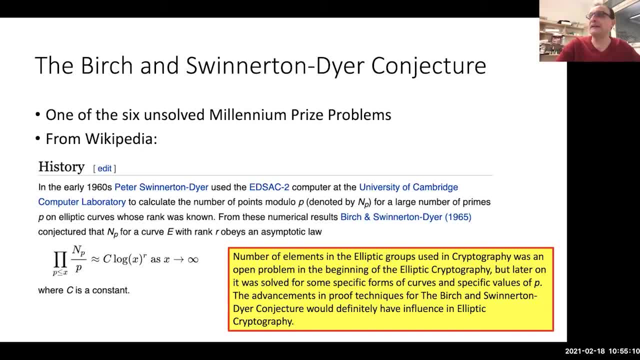 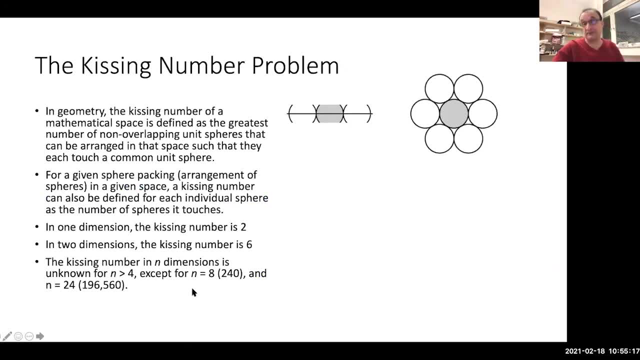 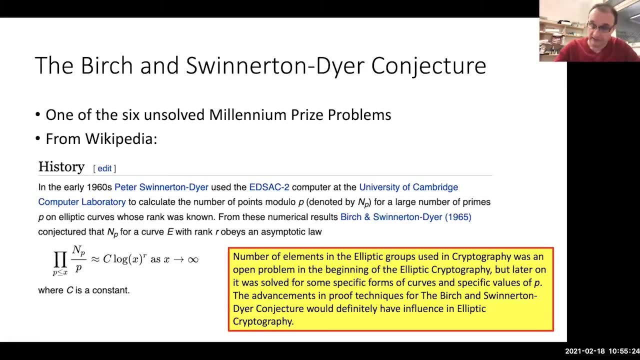 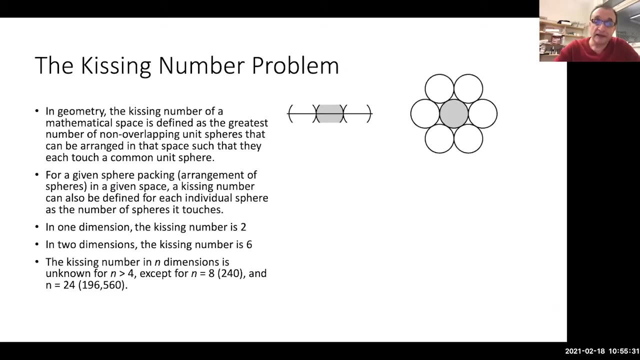 and for specific values of p, and for specific values of p and for specific values of those elliptical curves. So for general, this would be really a big advancement if this problem is solved, or new knowledge is gained from solving this problem. Then next problem: 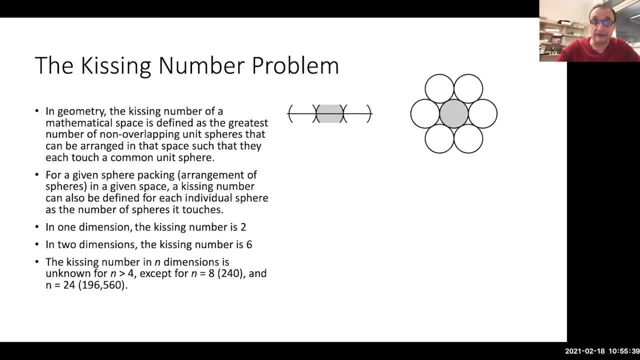 the kissing number problem is coming from geometry but also is very closely related with the coding theory, And it's given a sphere packing. basically, what is the number of touching points in the optimal number of touching points if you optimally distribute the spheres? 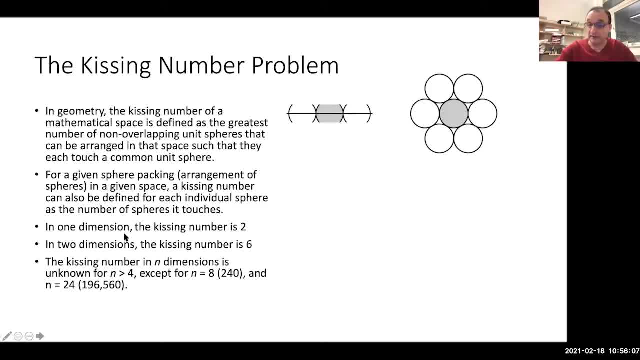 in different dimensions, And the answer is known for a very limited number of dimensions. dimension two in two dimensions. in one dimension it's two in two dimensions it's six, And for all dimensions except for dimension eight and 24,. 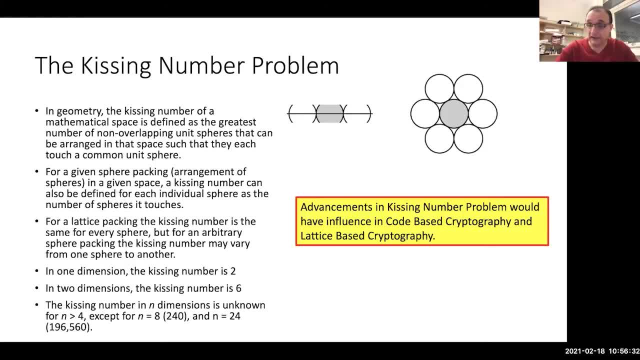 that number is unknown. So the advancements in kissing number problems will have an influence in code-based cryptography, in lattice-based cryptography, And these two types of cryptographies actually are nowadays a very serious candidates to offer algorithms that will be so-called post-quantum cryptographic algorithms. 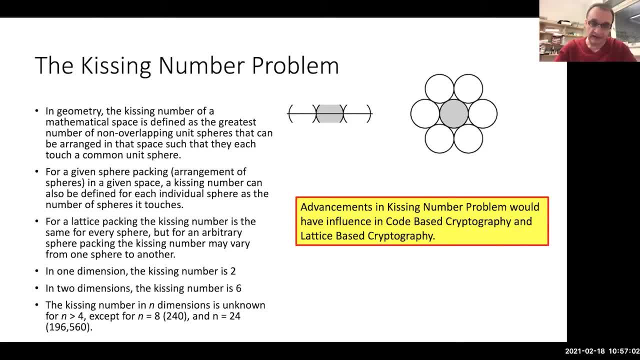 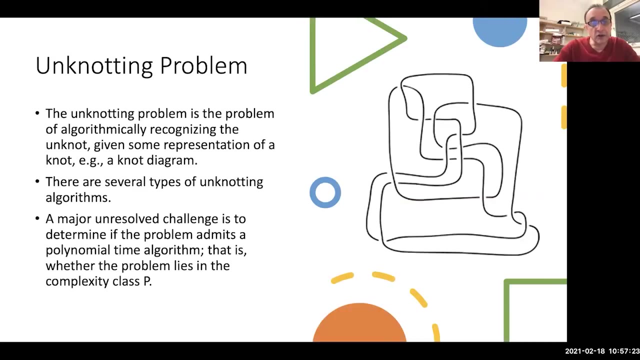 meaning when the advancements of the quantum computers is realistic, the current, the elliptical curves or RSA-based cryptography will be broken, but these types of post-quantum cryptography algorithms will be still resistant and safe. So another problem that also has an interesting connection. 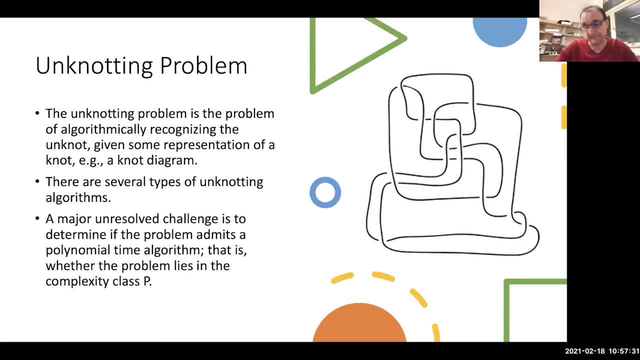 with the cryptography is the un-noting problem, And the un-noting problem is the problem is the problem of algorithmically recognizing the un-not giving some representation of the, not as the diagram, And this is coming from topology, but in connection with that. 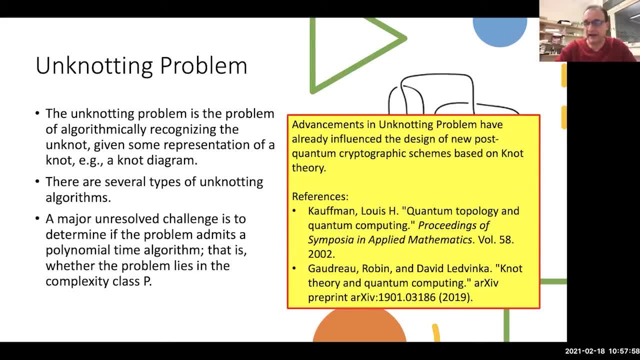 there have been bright groups and even the quantum topology and quantum computing And I just I just mentioned- and there is a nice advancement in that direction, but I just mentioned that actually advancements in the quantum computing thing is very much influencing now- the advancements in cryptography with these constructions. 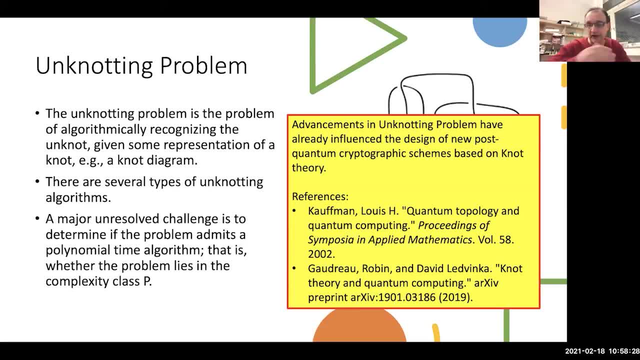 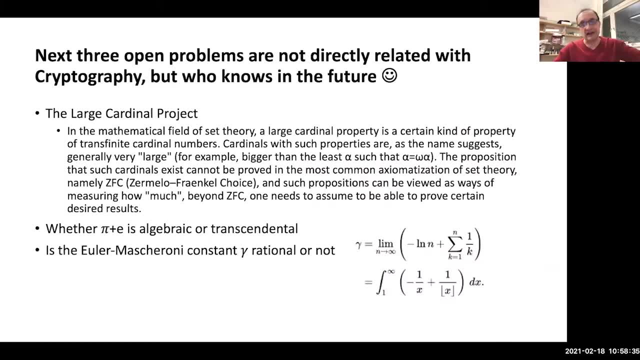 of post-quantum cryptographic algorithms, So it's really nicely connected. Well, next three problems are there in that list, So I couldn't find direct connection with cryptography. but yes, and anyway, I read this, but because maybe someone from the audience is working. 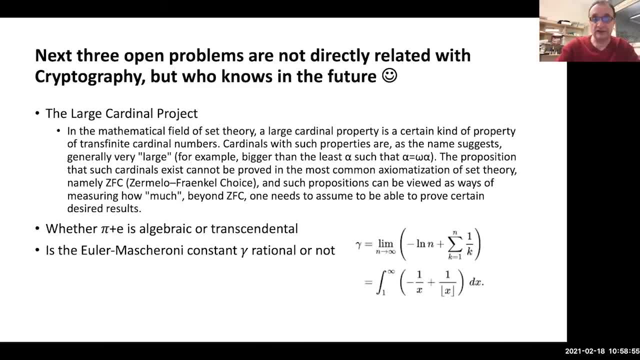 in that discipline, large cardinal projects. So a large cardinal property is a certain kind of property of so-called trans-finite cardinal numbers and which are the numbers sort of like axiomatic setup or axiomatization of the set theory Zermelo-Fraenkel choice. 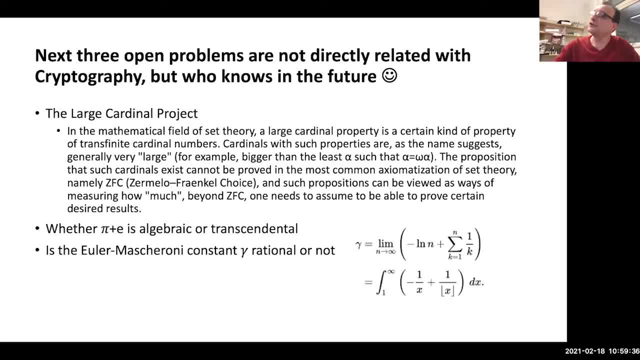 And this, probably these notions of infinities like Aleph zero, the simplest infinity, and more and more and more complex notions of infinity. I don't know is there any direct connection with cryptography, but at least this is interesting and open problem. 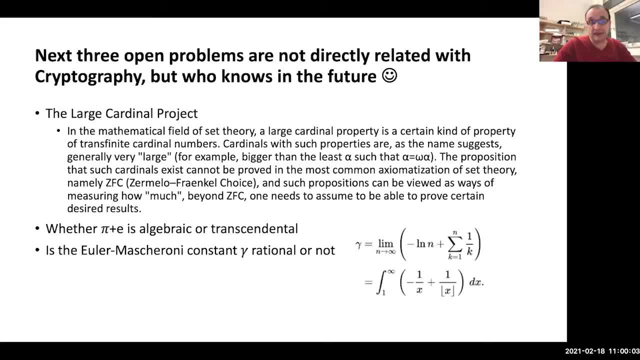 Another question or another problem is: is P plus E algebraic or transcendental Direct connection? I don't know, but it is interesting problem. Or Euler, or Euler-Mascheroni constant, is it rational or not? So if you sum up all natural numbers, 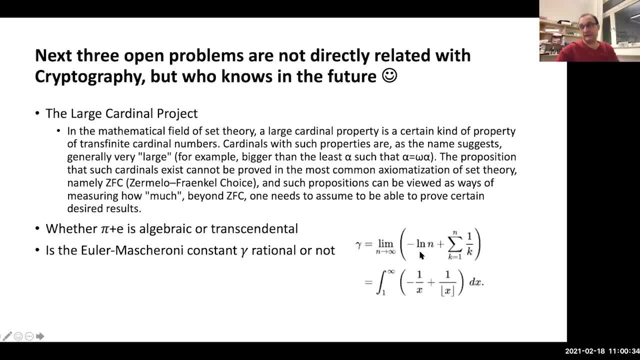 the inverse of all natural numbers and divide minus a logarithm, natural logarithm of N. when this N goes to infinity, is it rational or not? No one knows. Okay, so this is a summary of this, at least the first seven, and how they are connected. 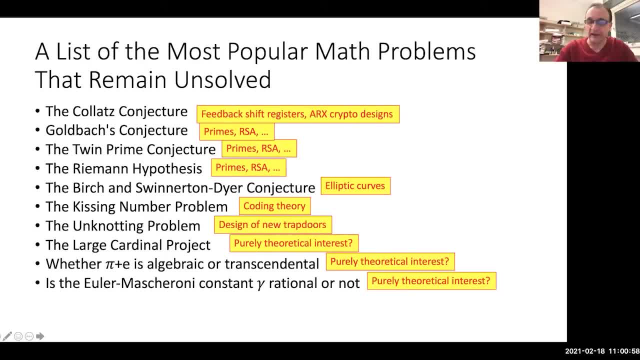 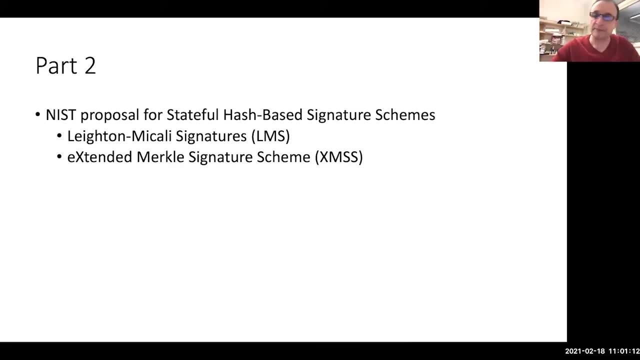 then the other three are: maybe they are pure theoretical interest, but you never know how you can make a connection, Okay, With some applied field like cryptography. Now I will briefly mention now something which is pretty much really specific for cryptography. 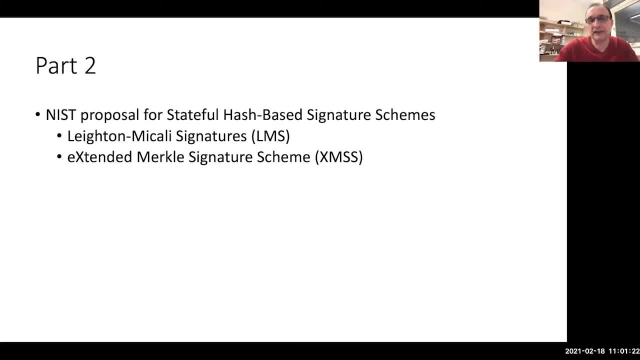 And this is this misproposal for stateful, hash-based signatures. So if you are lost in a lot of technical things, I will try not to go too deep into details, but just to give you, give you a flavor. Okay, How it is contracted. 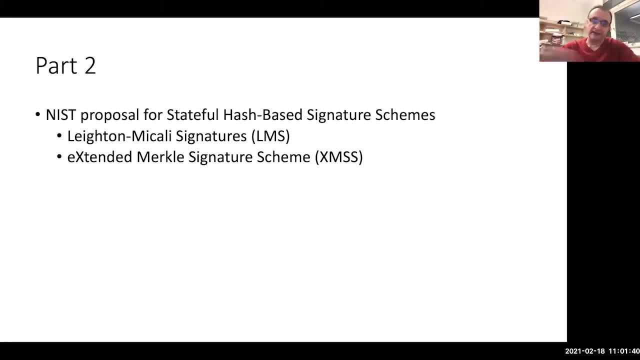 what are the intuition or intuitive ideas behind this? and then make the third part of with connecting all three parts together. So what is this state of so-called stateful hash-based signature? So the idea comes from one-time signature systems, And what would that be? 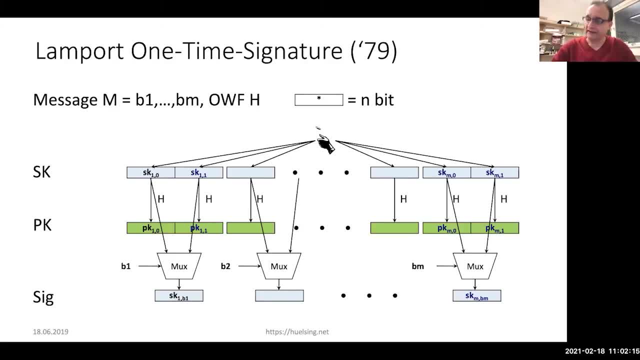 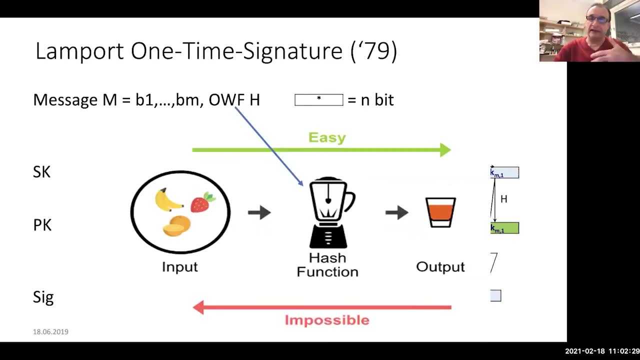 The very one ingredient that actually maybe you will find out easy to understand or intuitively understand is the notion of one-way function, So you can think of: okay, you have, it's easy to compute or to do computations in one direction. 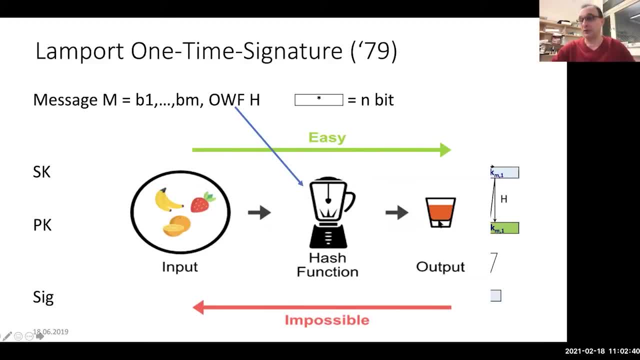 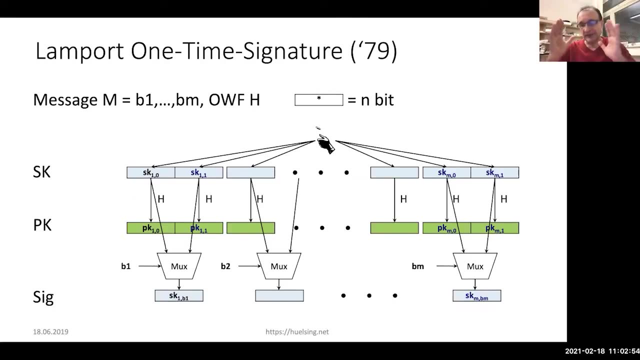 but once you have the output, if you are asked to return a back, it is infeasible or almost impossible. So that would be the intuitive notion. Now, from this intuitive, and there are constructions which actually are achieving that, No one has proved that one-way functions. 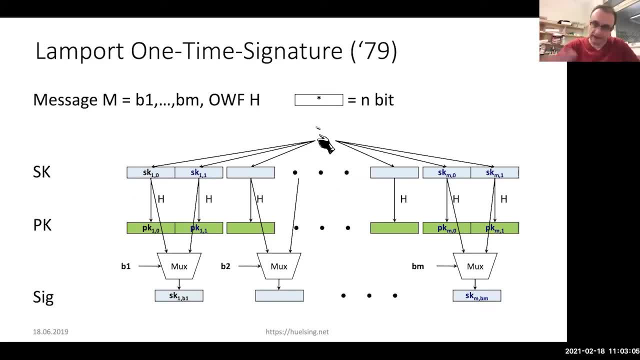 mathematically exist No one. So that is also one problem, open problem. No one has proved, but there are a lot of constructions that seems like one-way, without proof. Now, if you have such a construction, then the idea is produce some randomness. 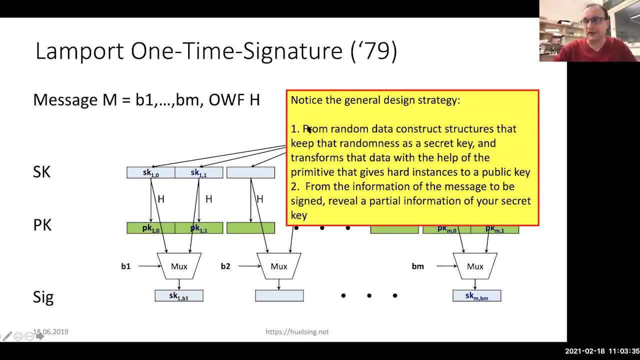 Yeah, So this the general design strategies: produce a random data and then consider that produce random data as something that you will keep a secret because you produced it in a random way. But if you transform it with this one-way function, whatever is produced here, 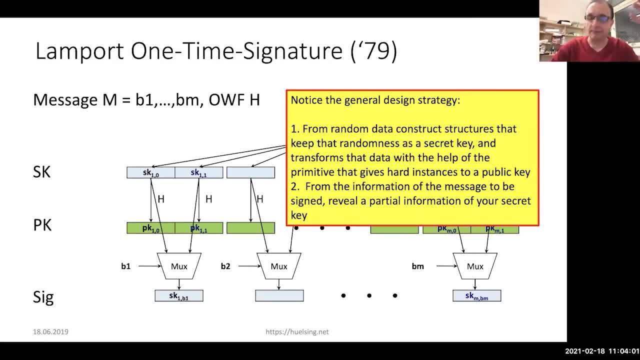 basically, you are allowed to give it as a public, public information. Why? Because you're relying on the hardness of this one-way function. If you give these green parts, no one can go back and find this yellowish parts. But that is. that is okay. one part. 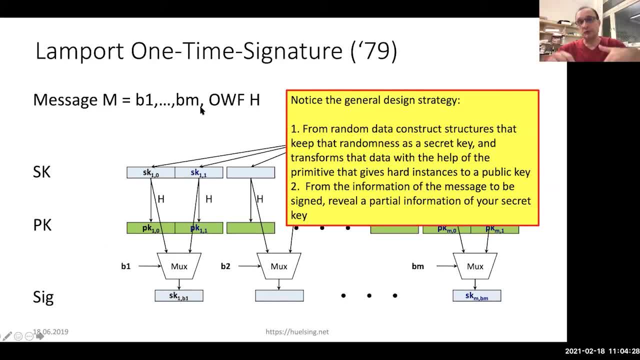 And then if you want to produce a signature, then you have to make a connection between a message and a public key and the secret key, And how this is done with this long time ago from 79.. Well, your message may be composed of zeros and ones. 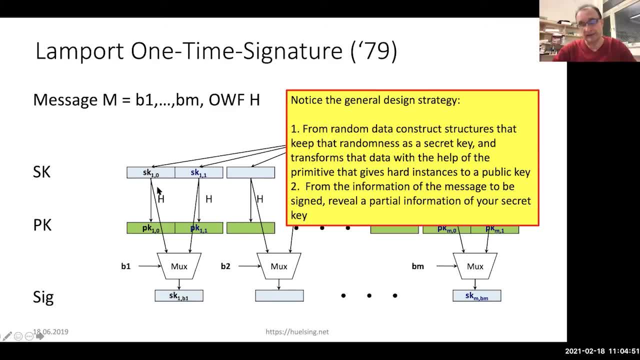 Since you produced a lot of randomness here. So for every bit, for the first position- this B1, your bit can be zero or one. For the second one, zero or one For one, et cetera. So your randomness can be here. 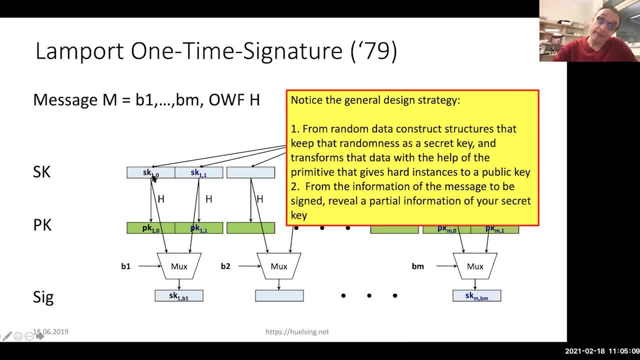 That is your secret. for the first bit, Maybe it was one, maybe it was, maybe it was zero, maybe it was one, et cetera. But now you would take this. So you will, just because everyone has this green part. 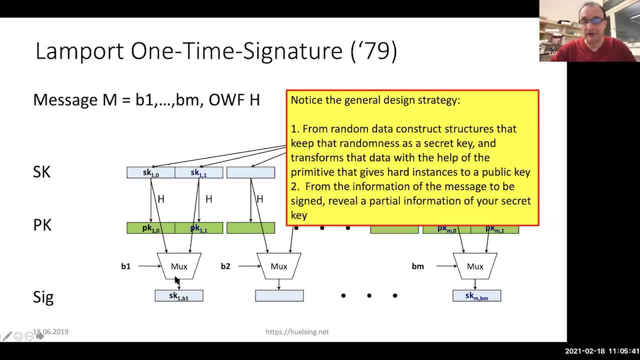 which is the public key, you will reveal just one part of you, either this part or this part. So by revealing only one of these secret parts, basically, and you are giving the giving the recipe, how you reveal it? because it was either zero or one. 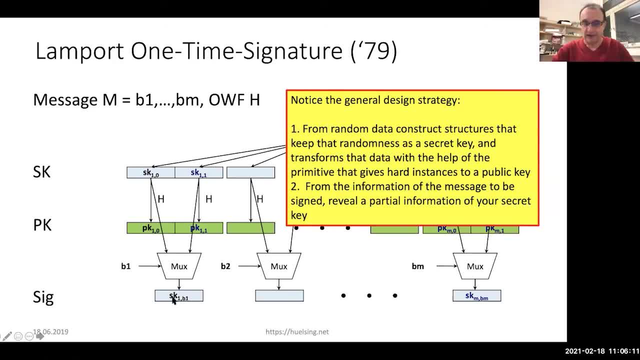 The verifier can take this revealed part here. make once more the hash function and check: is this revealed part actually giving you either this one or this one? if it is true, So the verifier will be convinced. wow, this is really incredible. It's really in connection. 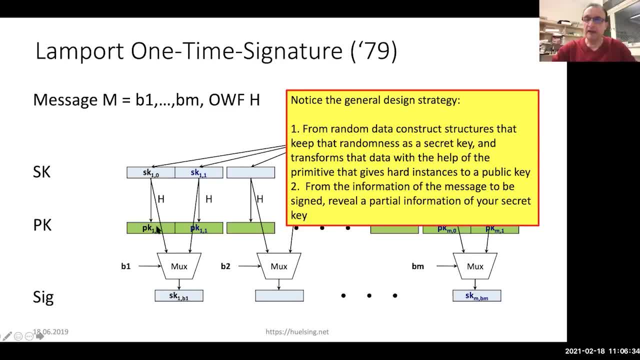 This message with this public key, really is in connection with the one that possess this secret parts. So that is the in general idea. I will not really go deeper because then suddenly it's become deeper. tiny little details that can can really make a big hurdle. 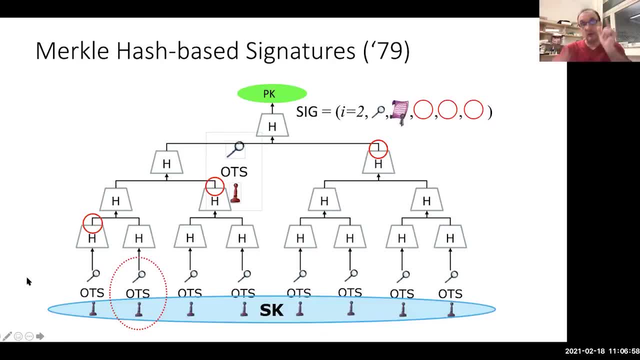 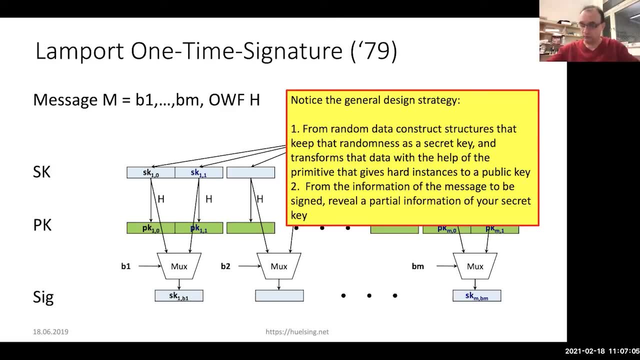 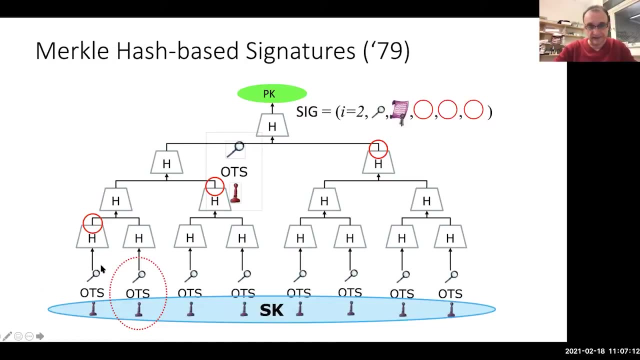 but then, but you can use this scheme only for one signature. In reality, you would like to make many signatures, So how you would do that? Well, the signature scheme, one-time signature- that I described here. imagine this public part. 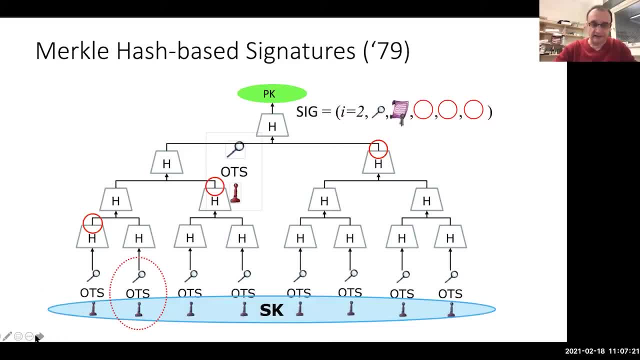 the big one, that you will hash it, And it is represented only by one leaf here. If you hash it, you have some result Which is represented here. Then produce another one, And that is represented here. Then produce another one, and another one, and another one. 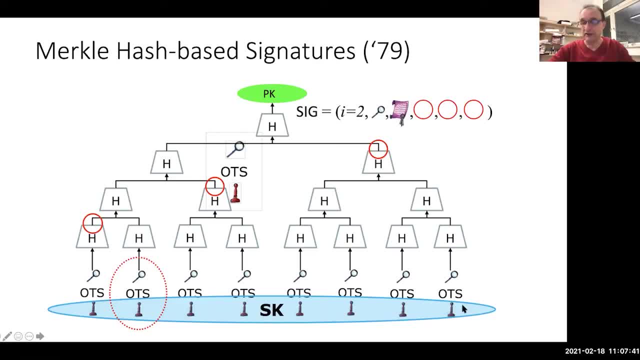 And then you say: okay, all these are one-time hashes, but if because if you compose them in a nice way, then actually you can publish only the root. So the root is small, You can publish only the root, And whenever you are trying to. 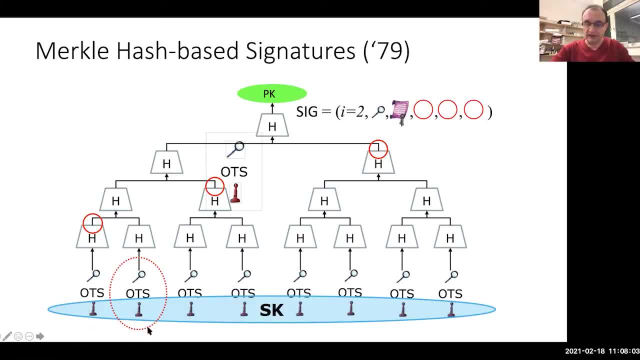 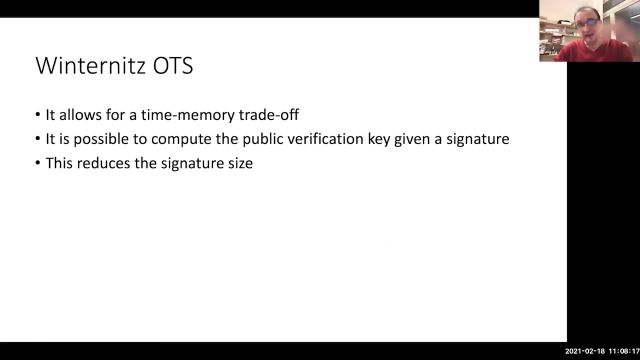 to make a signature. you will give the path to this root And because of the one-wayness all the construction is, many signature schemes suddenly because of this nice construction. And then there were several updates. I will not go really into detail because 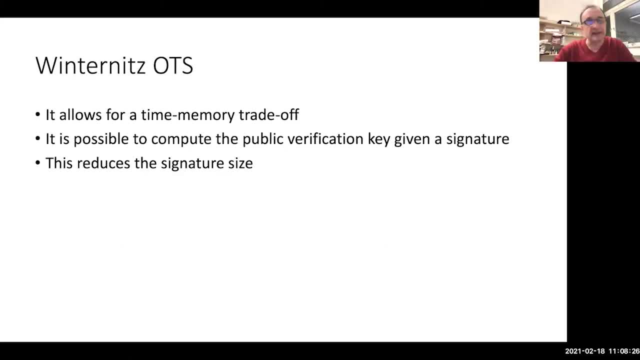 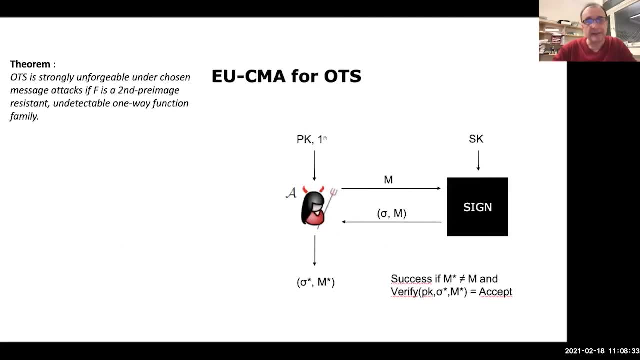 but one nice update or improvement of this was the Winternitz one-time signature. These details we will skip. These are also the details that actually that nice signature can be nicely and mathematically proof under certain assumptions that actually is really secure. 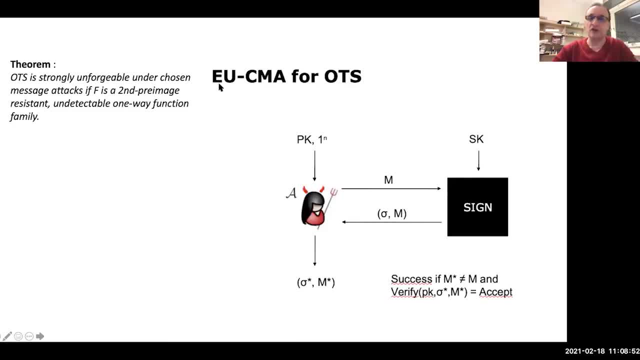 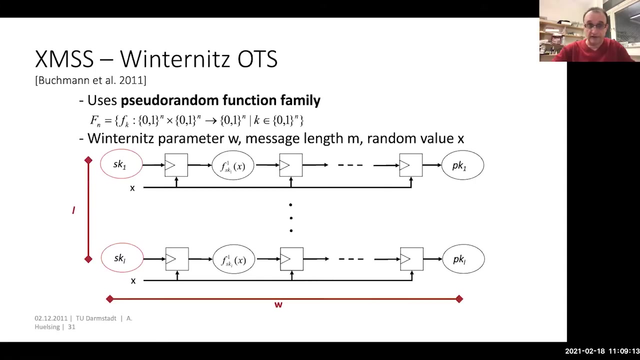 This is the abbreviation of existential unforgeability, with the chosen message attacks. So this one is mathematical, The mathematical area, very serious. cryptographic and mathematical modeling was proven that this is solid, This is nice and secure. And then, if you recall this idea, 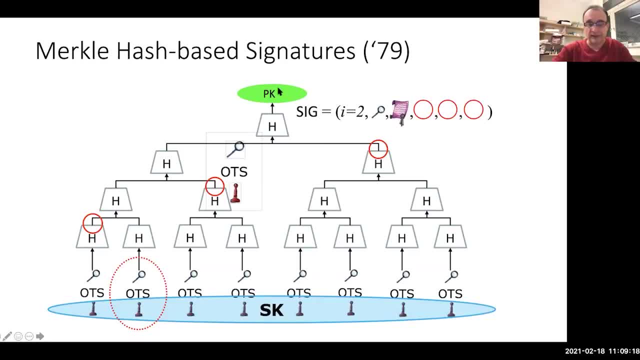 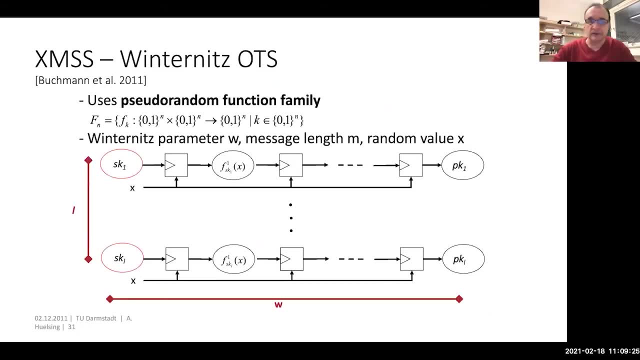 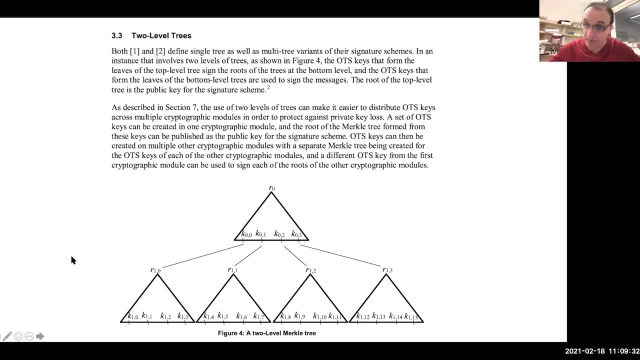 of combining some smaller structures into a bigger one, into the tree structure. it was even further. You can build even bigger trees of all the, all those other schemes into up even bigger schemes. And these actually compositions are the subject of this latest standardization that NIST is pushing. 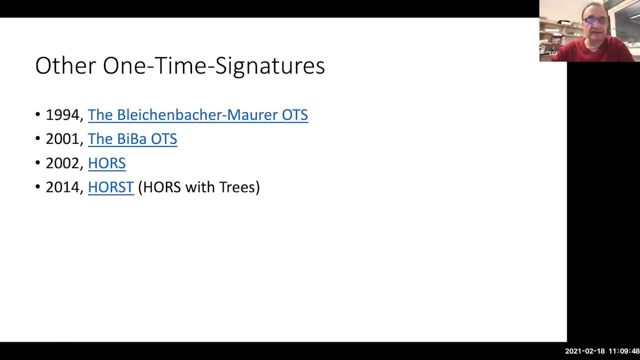 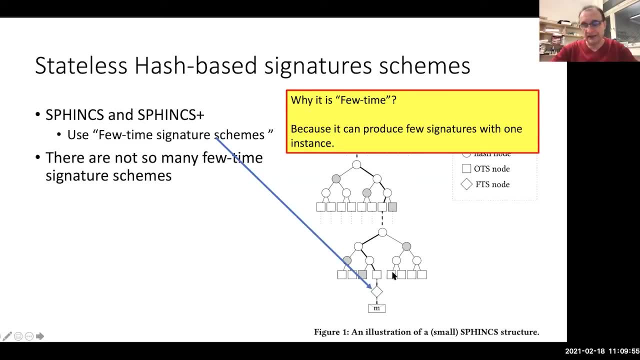 And there have been several similar flavors of this And, as you notice here, this combination of these of the one-time signatures into bigger structures. recently there was an idea, Okay, but why? There is a strong argument why the schemes that I. 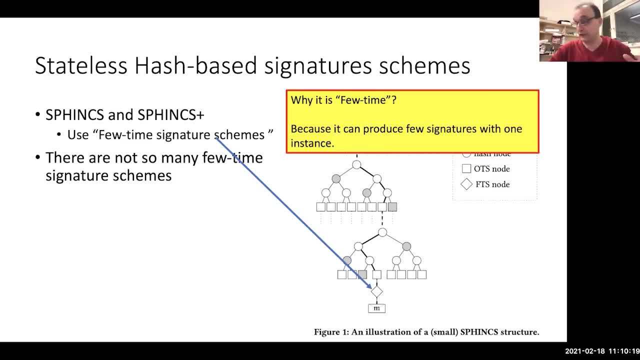 in the beginning I mentioned why it's only one-time signature, because if you use it once more, basically you will reveal a lot of previous. you revealed some of these, So basically, you are, you are not, you are not, you are not. 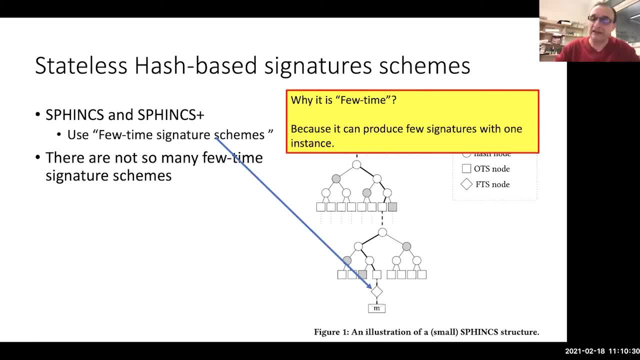 you will have a lot of machines. you will have a lot of machines revealed some of the secret key and then you're basically you're leaking uh, yours, uh, too much of your secret key. so that's why it's one time, but uh, in order to make um, uh, these schemes. 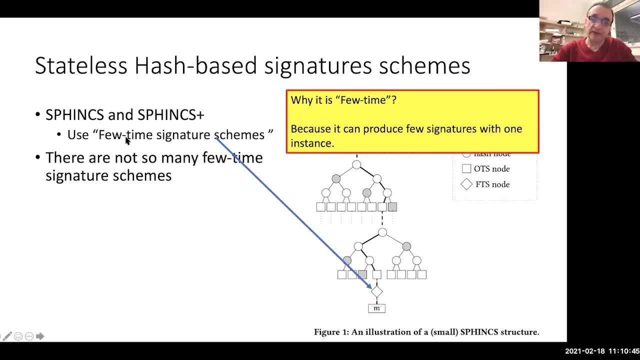 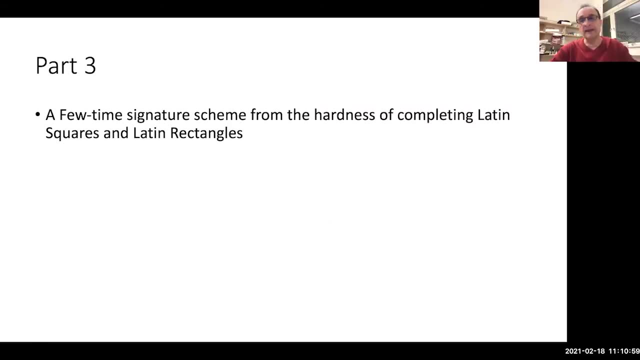 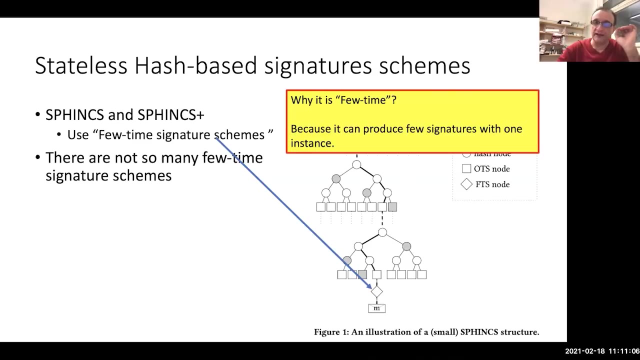 more efficient in size. people came with a few time signature scheme. and why this few? because you can use it for several times in uh, until uh it's uh too much use, and then you have to uh go for for our next one. now, um, how can we actually um, can we go through this uh through? 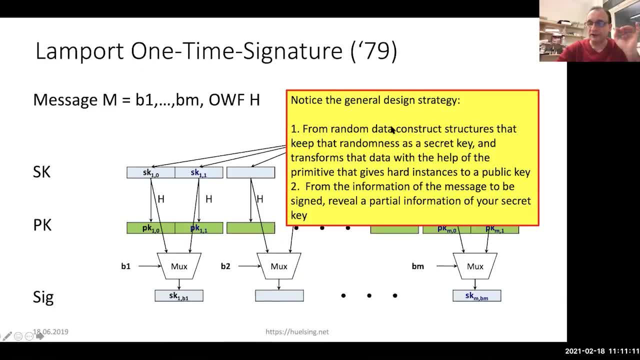 this uh recipe here from a random data, construct structures that keep that randomness as a secret key and transform that data with the help of the primitive that gives hard instances and from the information of the message uh, to be revealed the person. if you have this recipe maybe also in your mathematical area, where 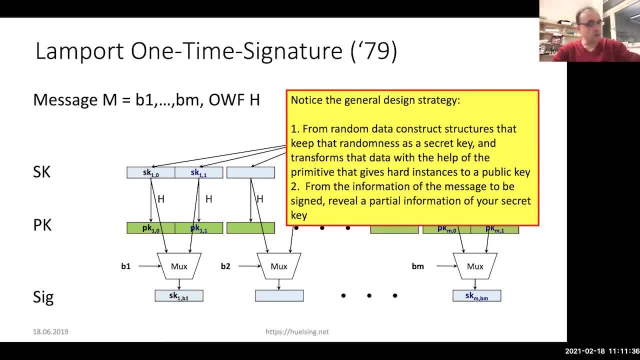 you know, oh, this is a hard problem, but this problem can do something else. i mean, it's not about one-way function, it's not about uh, but maybe it's in in your mathematical area. but there are some problems which are hard to solve and you can actually. 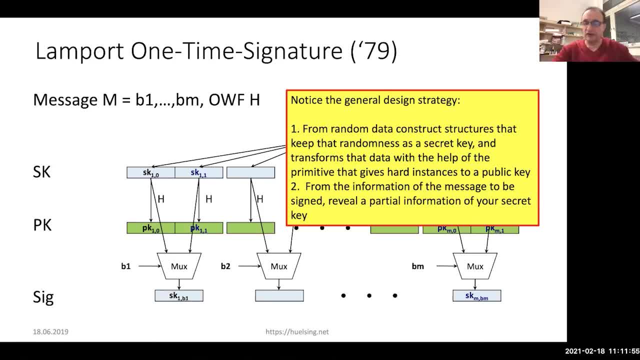 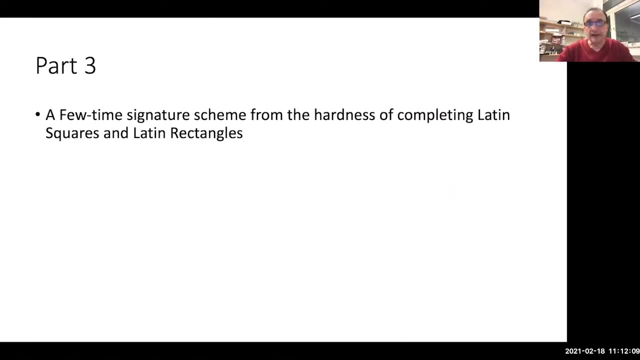 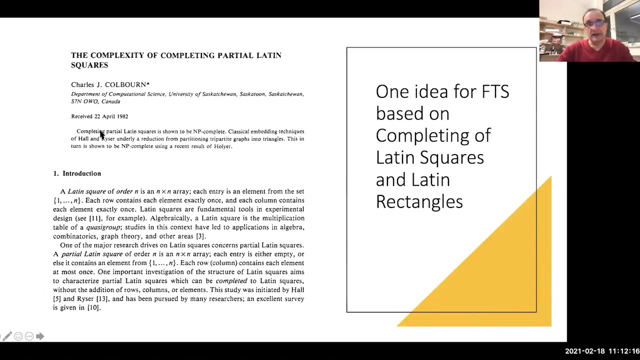 construct, uh, with just generating a random data, you can construct objects which, uh, you can transform through that hard problem that you are working on in mathematics, and this is that connection. so in the combinatorics, uh, there is uh one hard problem. uh, basically, it was shown that this actually 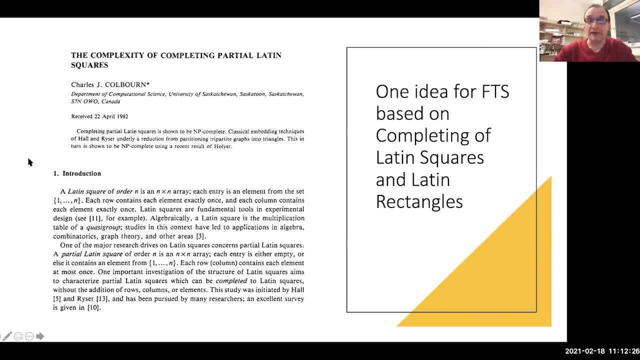 complete problem. so if you have a partial latin square, latin square uh, probably you know, are the um squares where all the columns and all the, all the rows and or all columns consist of n elements different and elements, permutations, um. but if you have a partial uh, meaning uh, that uh, you. 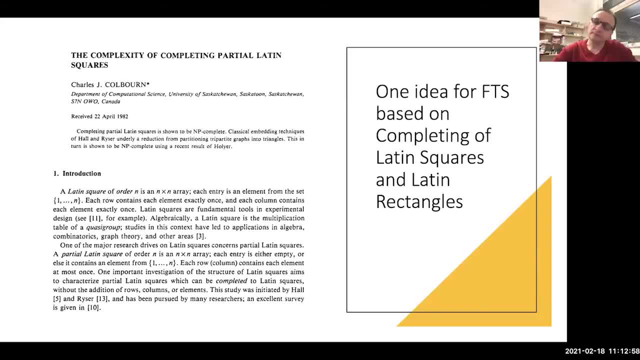 you construct one and then remove uh uh elements and basically uh uh. then the, the, the square is sort of like with empty cells, completing that uh uh, that uh partial latin square or latin rectangle is mp complete problem and there is a nice um proof of that effect. 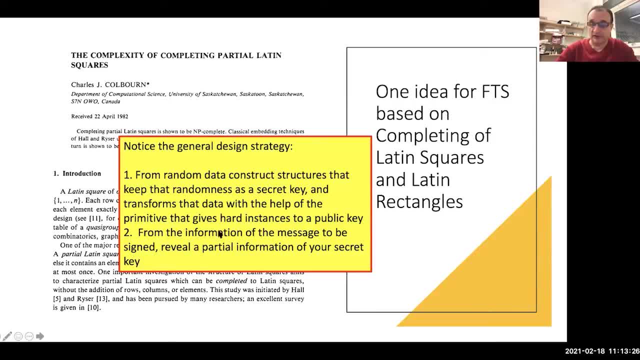 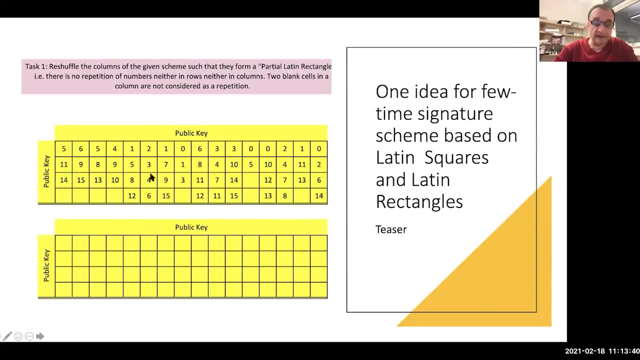 uh, now again. this was the recipe previously, but for another structure. but can we apply the same recipe here? uh, uh and now, um, i so probably, uh, once i produce, probably i will. i will give uh, uh. these slides as a pdf. you can try for yourself. having only these two, 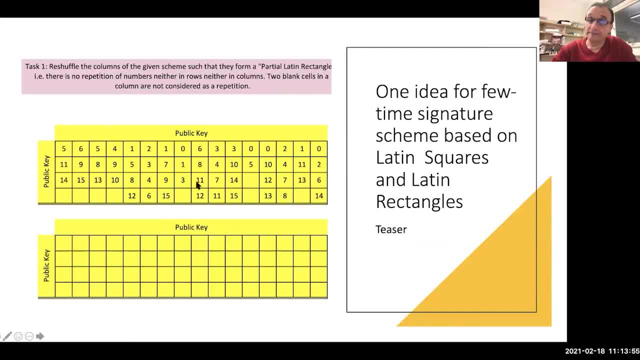 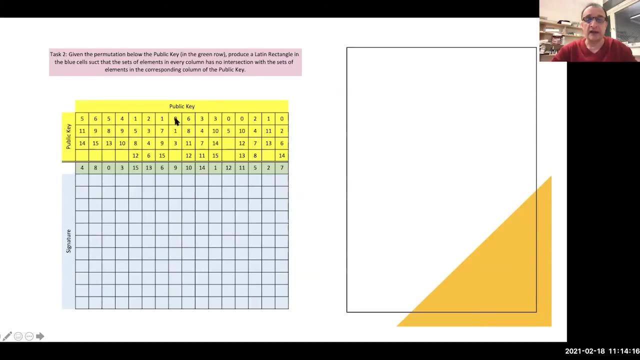 this sort of partial Latin square, Although this one is not even a Latin rectangle, because basically these have been, these have been kind of reshuffled and you can see here zero and zero is two times, but you should find out the proper position of zero here. 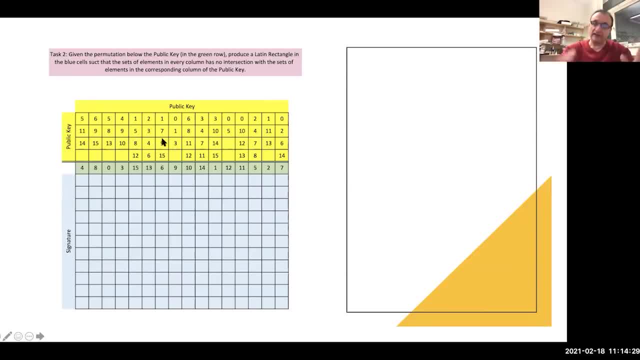 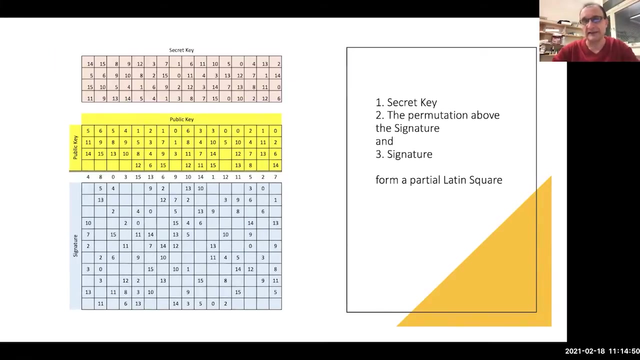 and zero here in order not to repeat, And everything is coming from really a partial Latin rectangle. Now, having that partial information which can be given as a public key, how can you produce signatures? Now, I will give this in general. So we need for all the ingredients. 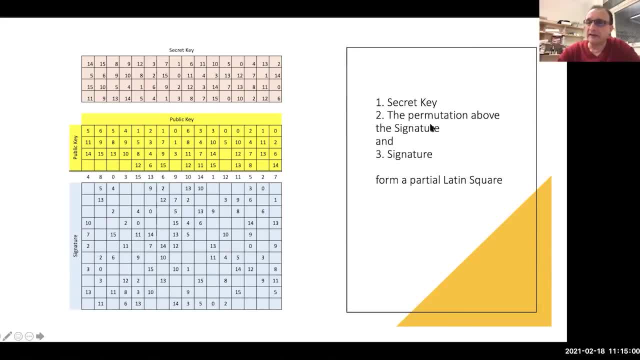 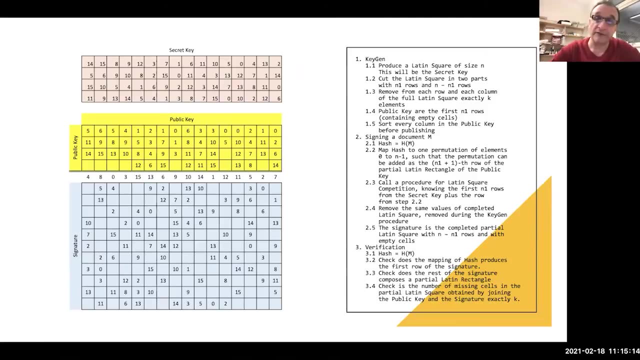 from the public key cryptography. we need a secret key production of secret key productions of signatures and verifications of signatures. So basically, in a most strict cryptographic recipe, this would be that you need a key generation procedure, you need a signature procedure. 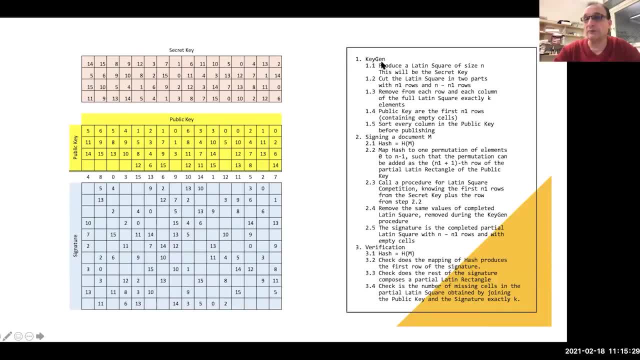 and you need a verification procedure And key generation procedure would be produced a Latin square size M. cut that Latin square in two parts and one rows and the rest remove from each row and each column exactly K elements. You publish the first part as your public key and 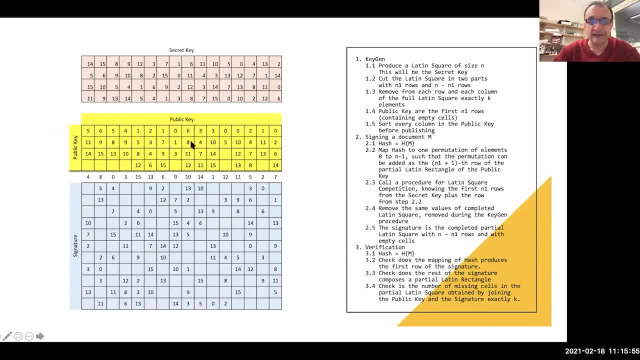 but you sort in ascending order And that is your public key And the knowledge of the whole Latin square and everything, or even just the first one rows, is your secret key And how you will sign. if you have a message, you will have to hash it to make a shorter one. 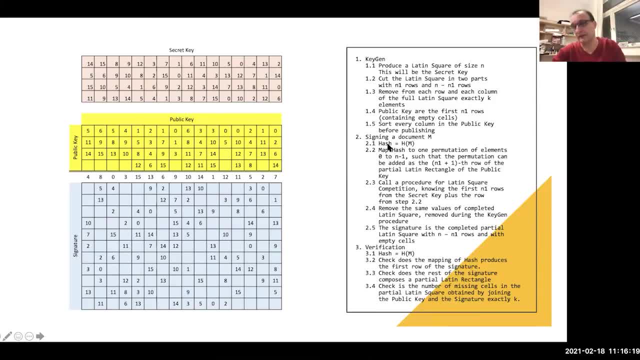 But out of that random, randomly looking hash value- there is an old algorithm here, reversal finding algorithm- map that random hash value to a permutation consisting of N elements in such a way that every elements does not consist of any of the public key elements in the columns. 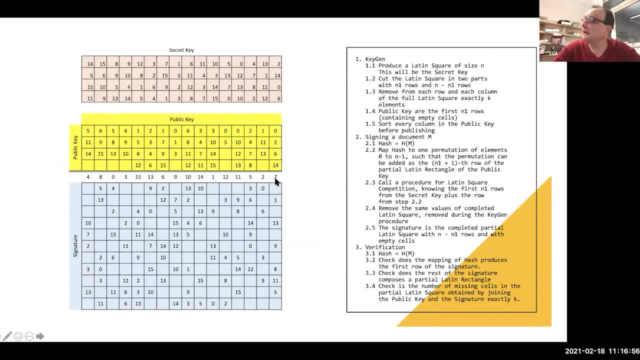 It's. this one is kind of like that hill routine is known from 60s or 70s within this Latin squares area of mathematics, And after that call the the same procedure but with the rest of the information and complete. 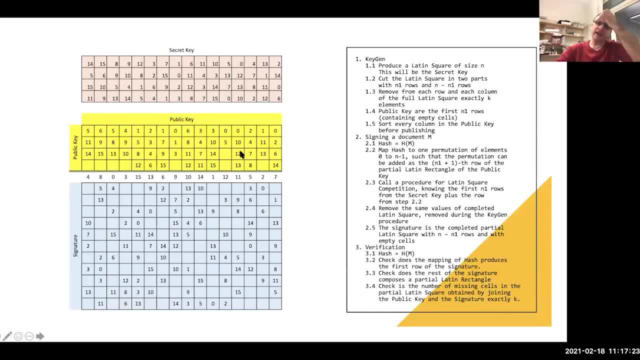 to the complete Latin square. If, since you know the secret key and the previous one, basically it's possible for you to to complete the Latin square, While for the rest of the public that have only this partial information, the problem. 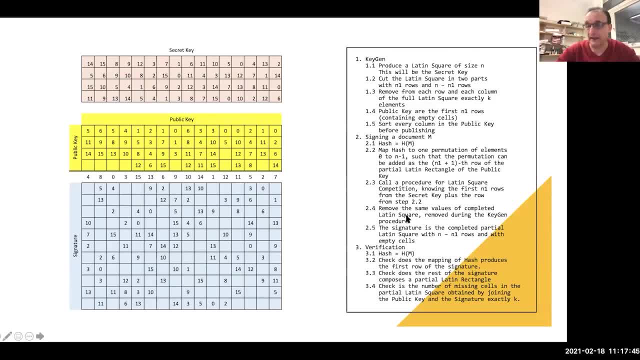 is almost like empty, complete problem, And that's the generation. So and then you publish this part and this part would be the signature And the verification would be make the again the message hash check: does the mapping produces really this first row. 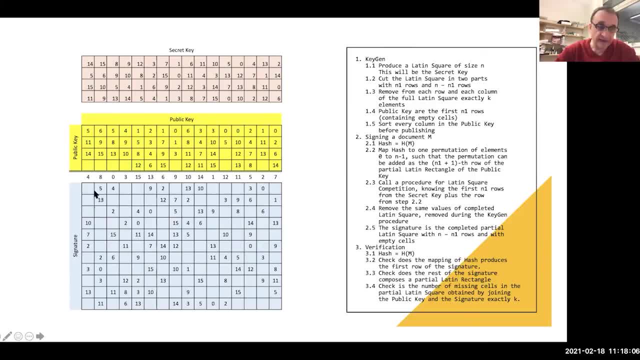 and then check if in every column and in every row there are missing K elements And why. this would be the few times signature, because actually you can produce few times with few messages. this row here and still not revealed too much for this missing elements. 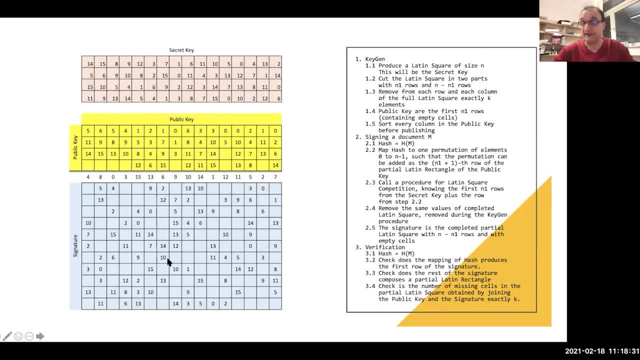 because, basically, these missing elements, once you reveal one signature, basically you are giving. you're giving not just your public key, which is partial Latin rectangle, but the rest is partial or complete. And so this is the problem: Completing is the partial Latin square. 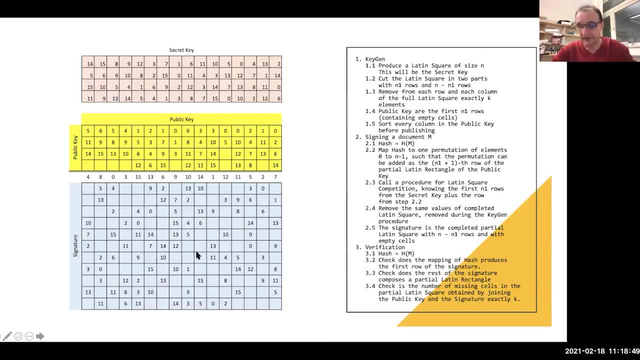 But completing that partial Latin square is hard. If you use it one more time, you will reveal some of these missing elements, but not all of them. Still, you have partial Latin square and that's still a hard problem, But you should not use it too much time. 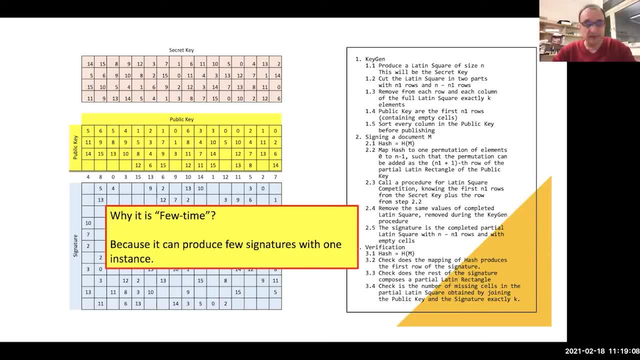 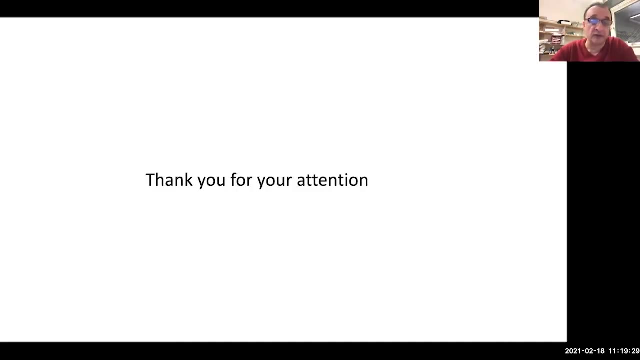 So this was why it is few times, because you can use it a few times. So this is the connection between one of the hard problems in combinatorics with the things that I was working in the past two years. So with this, I would like to thank you for your attention.